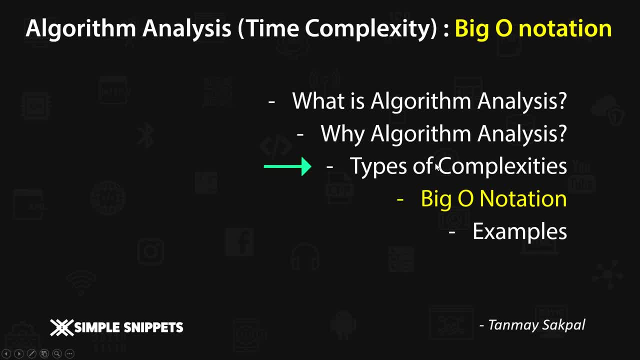 to be answered. After that, we are gonna be talking about the types of complexities and then focus on Time Complexity and, lastly, we are also gonna talk about Big O Notation by taking some examples. Now, before we proceed, make sure you watch this video till the end. 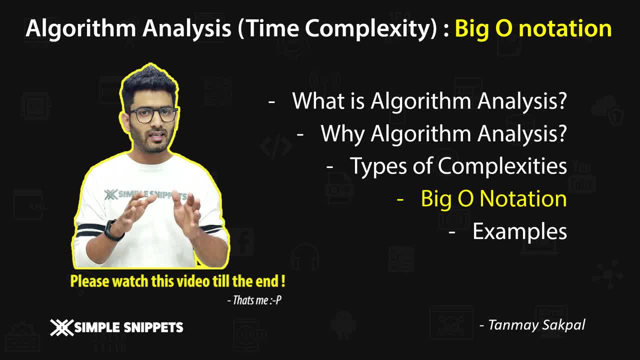 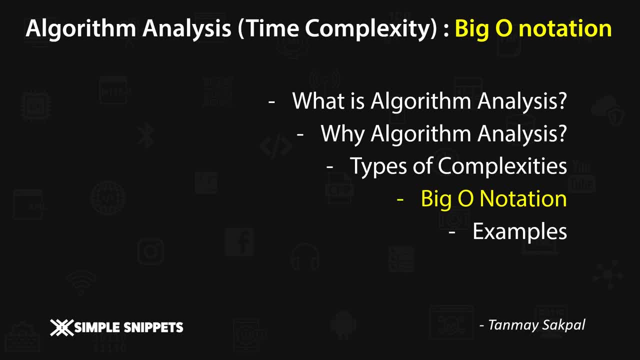 this is a request and I can assure you guys that by the end of this video, this topic of Algorithm Analysis and what is Big O Notation and what is Time Complexity is going to be very clear, and this is a very, very fundamental topic, very important when it comes to interviews. 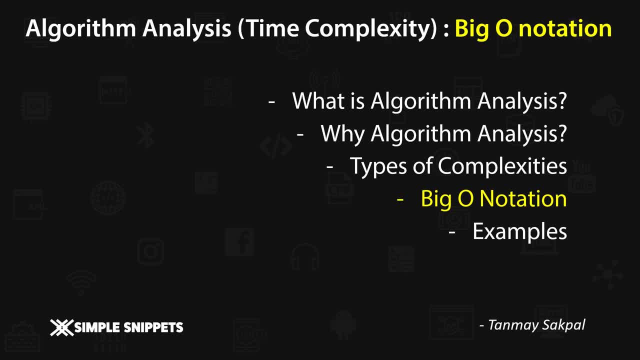 also and also when you are learning Data Structures and Algorithms. So please make sure you watch this video till the end. as I mentioned, I can assure you that I will make this topic very easy and by the end of it, you will understand everything and we will also take some practical 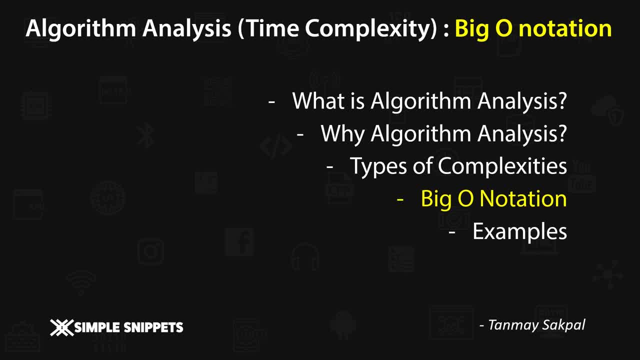 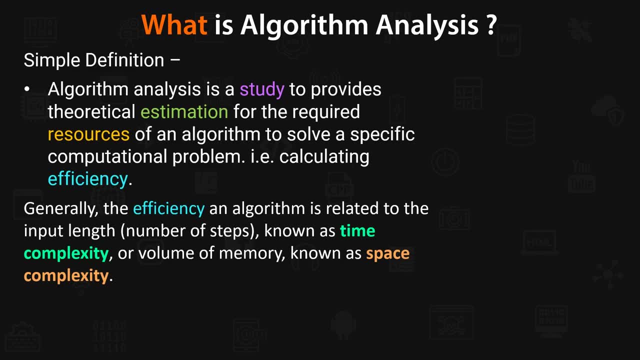 examples. so this is not gonna be just a boring theory video. Okay, so let's start off with what is Algorithm Analysis. So I am assuming that you already know what is an Algorithm. if not, we've already discussed that in this Data Structures and Algorithms course. I will drop the link in the video description to this entire course. 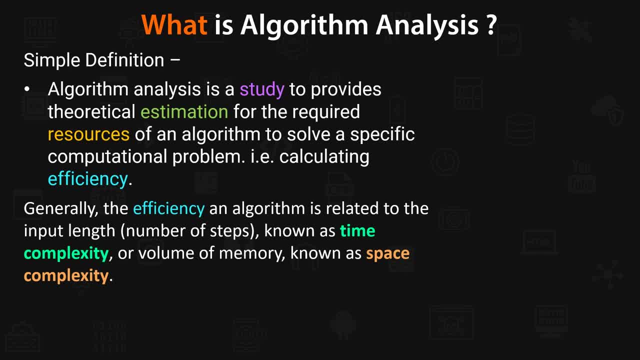 you guys can check it out. but then what is Algorithm Analysis? Now, the word analysis should already give you a little bit of hint, but a simple definition over here is: Algorithm Analysis is the study to provide theoretical estimations for the required resources of an algorithm to solve a specific computational problem. that is, basically calculating the. 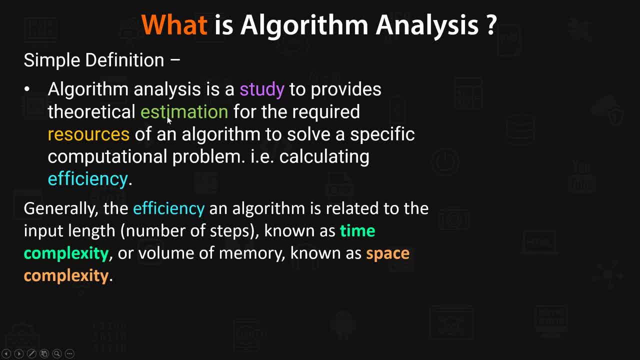 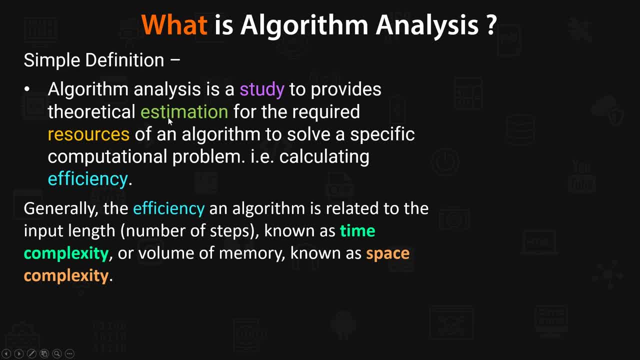 So when you put it this way, it makes sense. So, ultimately, an algorithm which is running on your computer, which is running in your PC, is gonna take up some resources. for example, it will take some memory, it will take some time to complete its execution, and these all 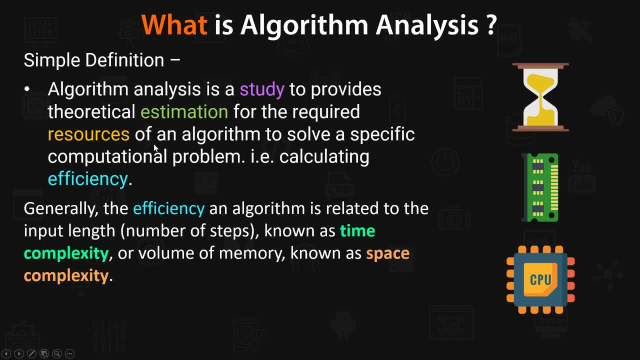 things are supposed to be studied in order to make some estimates. So algorithm analysis basically just helps us give some theoretical estimations. Now, the reason why I have highlighted estimations is because we do not get the accurate value, because to find out accurate value is very difficult, and that's why we can only make 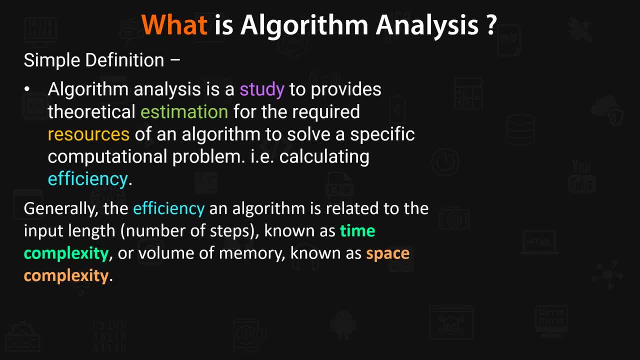 some theoretical estimations, theoretical estimations using this algorithm analysis techniques which, overall, gives us how the behavior of the algorithm will be, and we will talk about that in detail as we move ahead. So, as I mentioned, generally the efficiency of an algorithm is related to the input length. 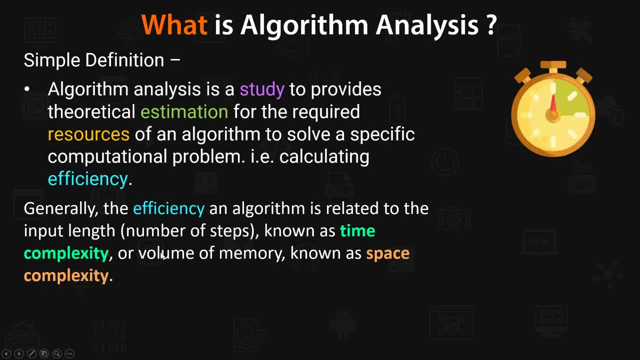 that is the number of steps, also known as time complexity, or volume of memory, known as space complexity. So it makes sense, right? if your algorithm has 10 steps, it would take some particular amount of time. but if that step increases, let's say it becomes 20 steps, obviously. 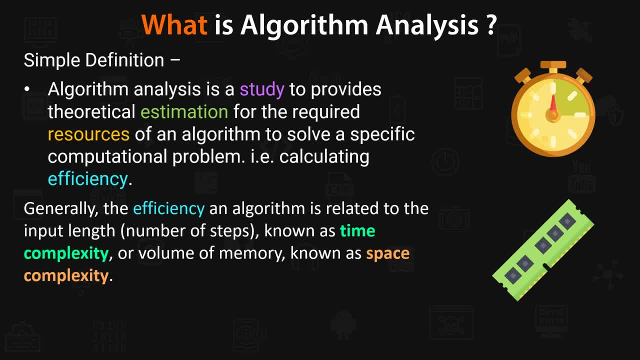 the time also will increase. So it makes basic sense, right and again, the space complexity also deals with how much memory your algorithm is occupying in memory when it is running. So whenever you are running a program it is occupying some memory in the RAM. So that is space complexity. So we are going to be focusing on time complexity in detail. 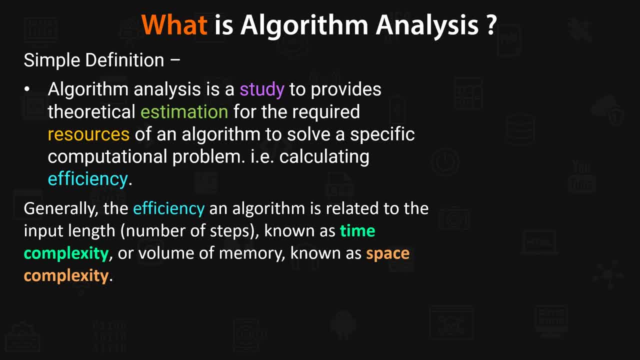 and we'll talk more, but I hope you've got a very basic idea of what is algorithm analysis. So, with this idea in mind- if you want, you can take a screenshot- Let's move ahead and understand why do we need algorithm analysis, because that is very important. So, when it comes to why do we need algorithm analysis, 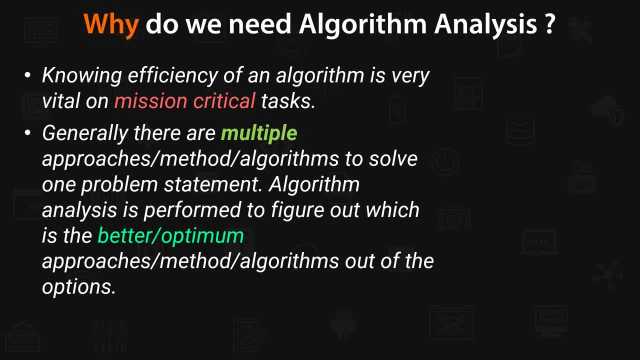 I'm going to put up two major, major points. So point number one, as you can see, is knowing the efficiency of an algorithm is vital on a mission critical task. So this makes sense, right, if you don't know how long your algorithm is going to take to execute or complete its execution. 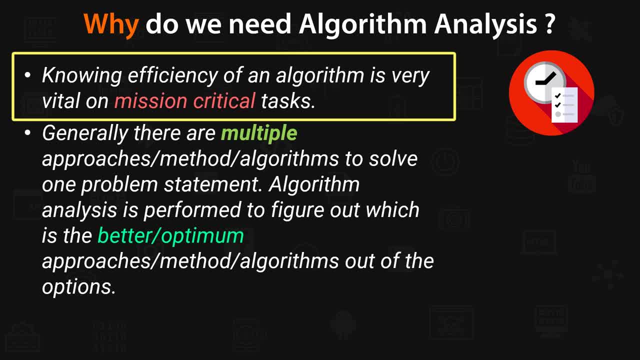 if your task is mission critical, then you might land up in some serious trouble. So to make it clear, let's take an example. Let's say you're working in NASA or you're working in ISRO or SpaceX and these companies basically launch space rockets and satellites into space, right? 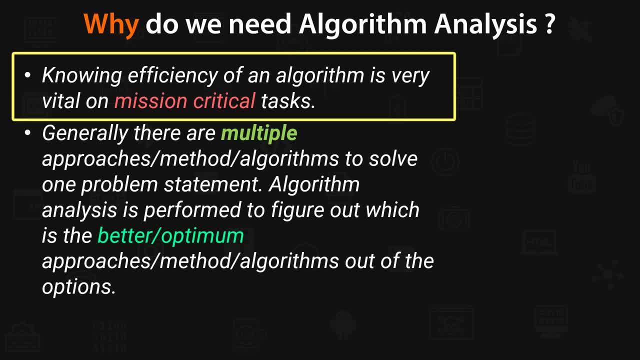 So let's say you're writing an algorithm or writing a computer program which is basically going to take this rocket into orbit and release the satellite at a particular height and when it reaches that height you basically have just 10 seconds for the rocket to eject the satellite. 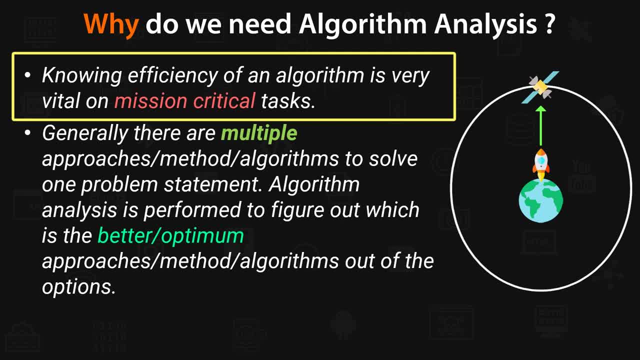 okay, So this is the problem statement, and now you need to write a program. If your program takes more than 10 seconds, your rocket will not eject the satellite at the right moment, right, And the satellite will get lost in space. Now you can understand the gravity of the situation, right? 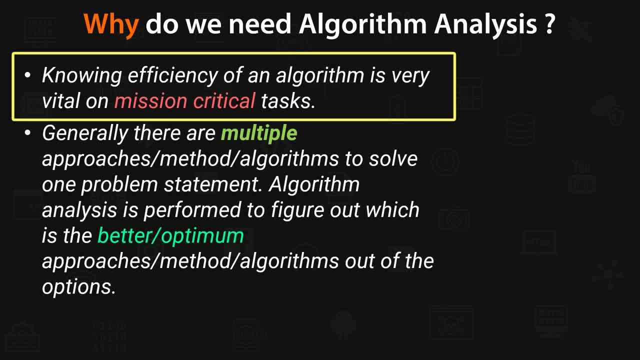 The seriousness of the situation. If your rocket ejects the satellite too early, it might fall back due to the gravity, And if your satellite is ejected after 10 seconds, it will get lost in space. So you can see how mission critical this task is, that you have to execute your program. 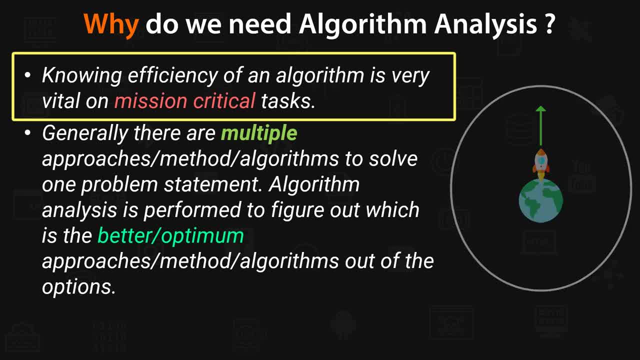 under 10 seconds only. So 10 seconds is your maximum limit. So that is the reason why you need to know how much amount of time your algorithm will take, or at least have a rough estimate about the maximum time right. Another example can be the ejection of airbags in a car. 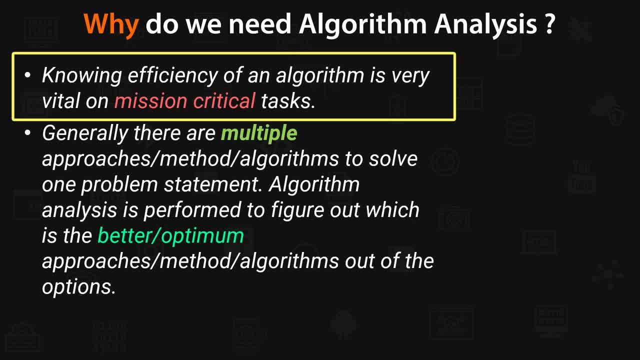 So nowadays, cars are equipped with airbags, So whenever you meet with an unfortunate accident, these airbags eject and they save human lives. Now, obviously there must be some algorithm which is written behind which detects that there is a crash happening or there is an impact and then it ejects those airbags on. 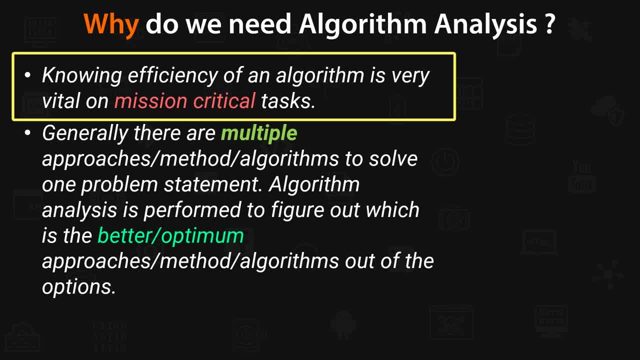 time. Now imagine if that algorithm takes more than 2 seconds. Now accidents happen in like less than 1 second right. If your airbags does not get ejected in time, a person's life might get lost. So this is a very mission critical task. 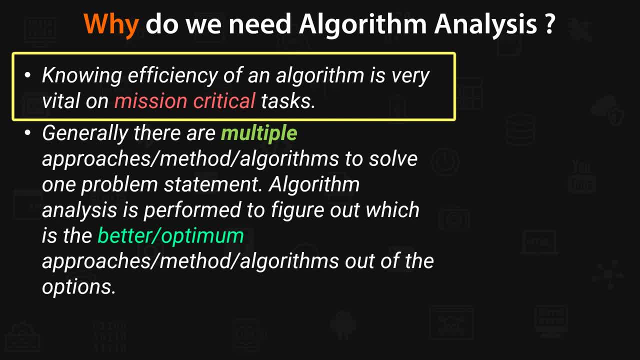 And hence you need to know exactly, or at least have a rough estimate about the maximum time the algorithm or the program would take to execute or complete its execution. So this was point number 1. And the point number 2 is even more important, or even more interesting actually. 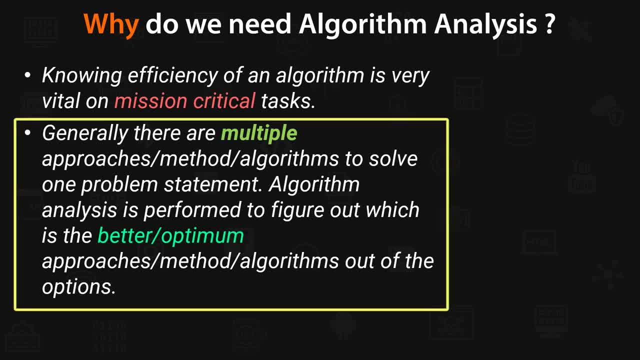 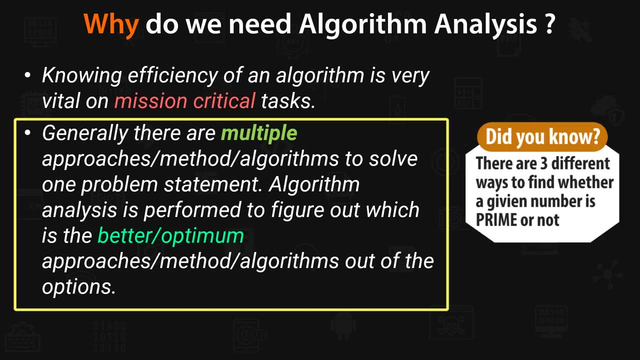 And that is Generally. there are multiple approaches or multiple methods to solve one problem statement, So algorithm analysis is performed to figure out which is a better or optimum approach out of the different options. for us, For example, there are three different ways in which you can find out. a given number is. 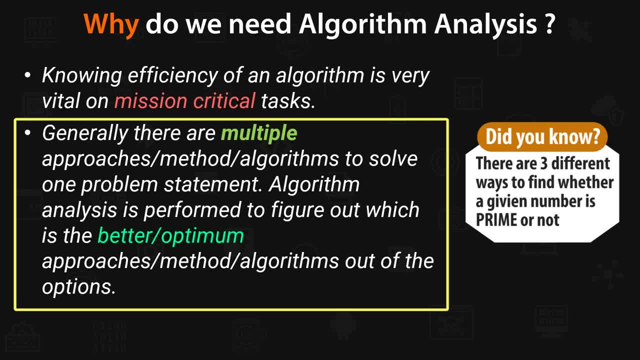 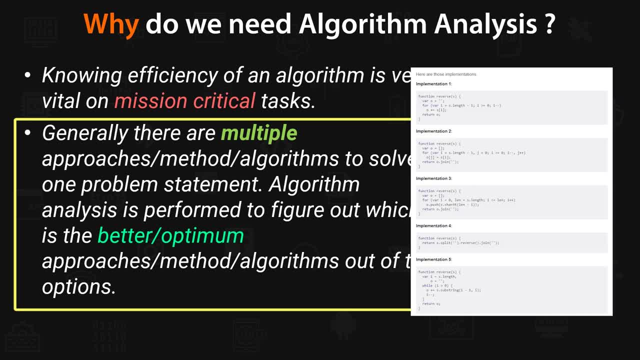 prime or not. You know what. you can just go ahead and Google it out and let me know in the comments below which is the most optimum. one Another example can be: there are like n number of ways in which you can reverse a string. 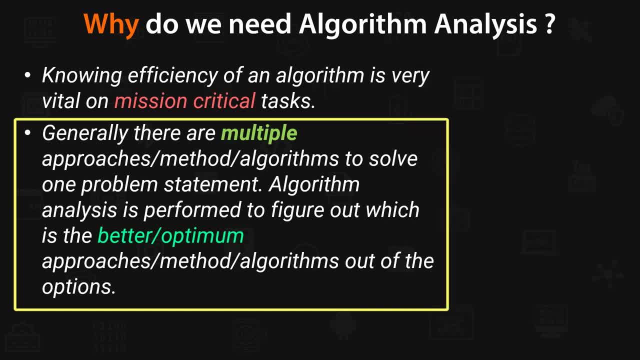 So all of them are different approaches, But they're doing the same thing And we are also going to see an example as we move ahead in this video, about an example which has two different approaches to do the same thing. Make sure you watch this video till the end. 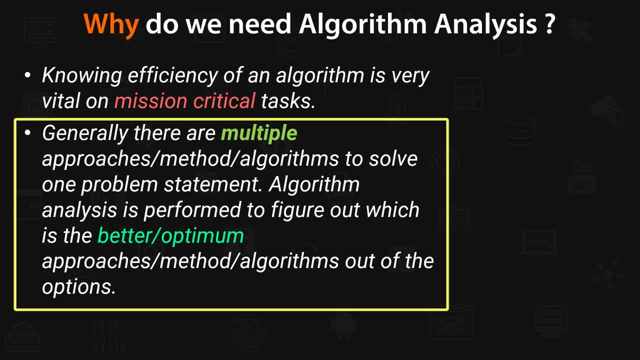 I know I'm reiterating it because it is very important And this video is probably the most important one in the data structures series, So that's why I'm constantly telling you guys to watch this video till the end. So I hope you're getting that. since there are multiple approaches, we need to figure 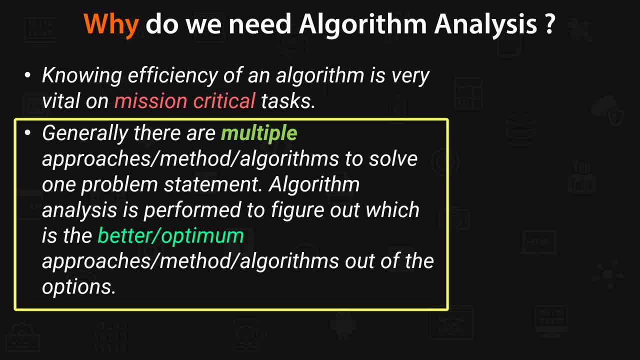 out what is the best for us, right? So that's why I said better or optimum. So when I say optimum, it does not mean the best. Let's say, for example: I have a computer system which has 10 GB of RAM and you have a computer. 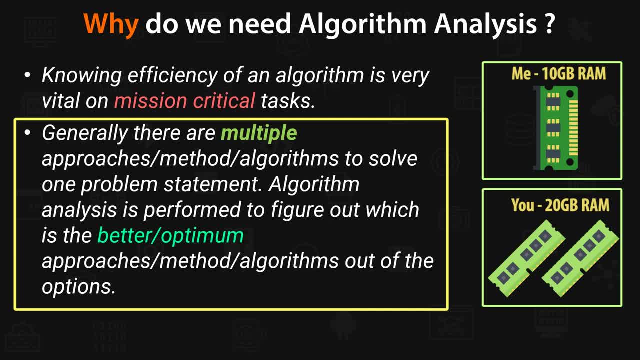 system which has 20 GB of RAM. Okay, we're just taking basic assumptions, So we both have the same task, But you can see that, since the RAM that I have is limited, my algorithm needs to be primarily thinking about the space complexity. 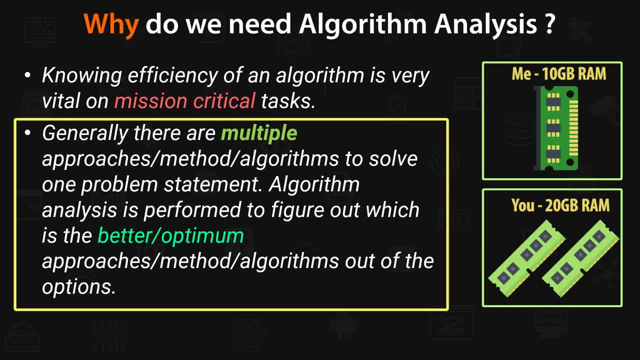 So maybe I can get away with a little extra time, but I need to save space. However, in your case, since you have so much RAM, you are not worried about the space. So what you are worried about is the space. So what you are worried about is the space. 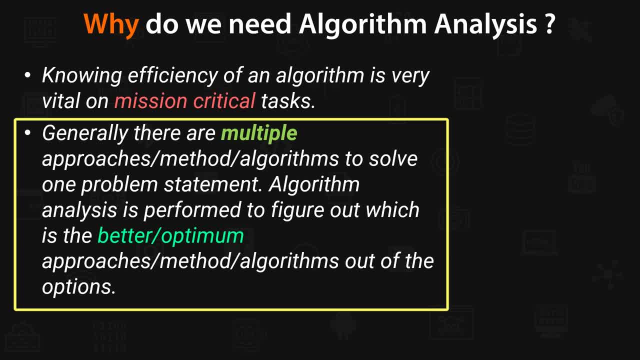 So what you're focused on is how fast can your algorithm run? So different situations require different criteria, and that's why, when you have multiple choices, you need to select the one that is best suitable for you. So these are two major reasons why we need to have a good algorithm analysis. 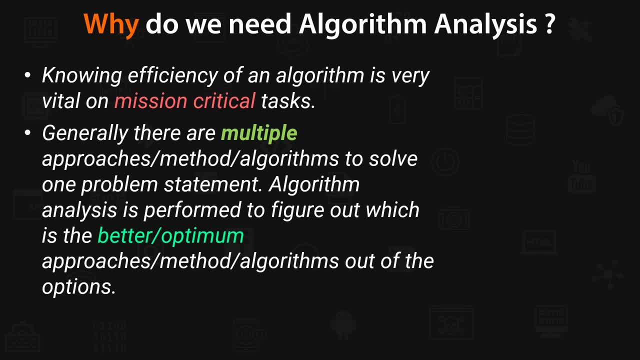 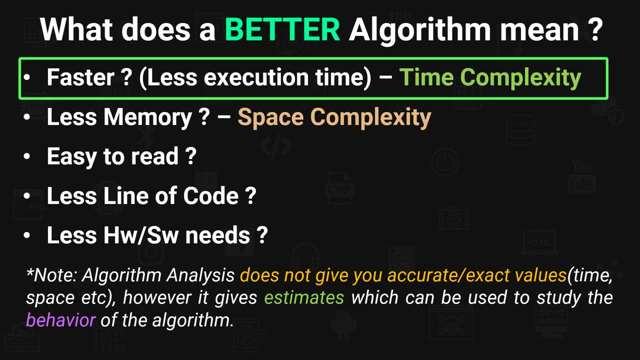 So, talking about multiple approaches, what makes an algorithm better? right, Let's, let's have a look. So the next obvious question arises: what does a better algorithm mean? Does it mean it is faster, which means it requires less execution time, and that's basically. 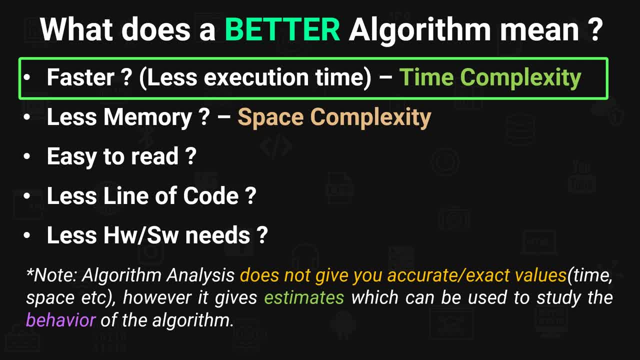 time, complex complexity- right, So we're also going to talk about time complexity more when we go to big O notation in this video. just hold on Now. another criteria can be less memory. Is your algorithm taking up less memory compared to some other algorithm doing the same thing? 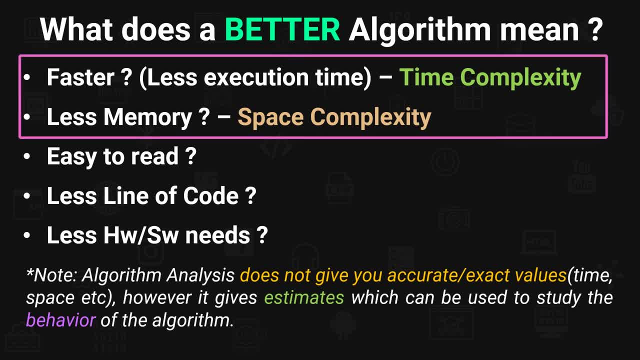 So that is dealing with space complexity. Now, generally these first two criteria are the most focused on, because those are the most important ones, especially the time. Nowadays our computer systems have lots of memory, so we don't really focus much on memory, but we are more interested in reducing the time. So we want our algorithms to run very 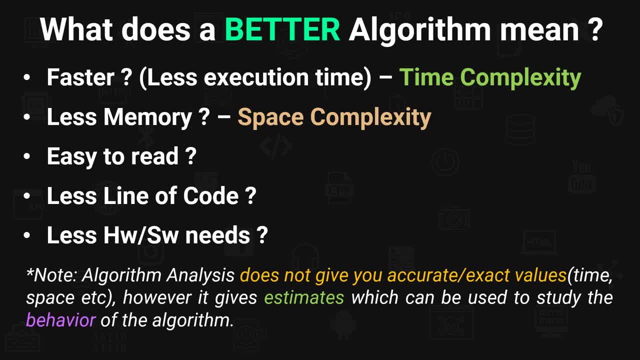 very fast. You don't want your website to wait like 10 seconds to load all the data. right, You want it in seconds. Now some other things that may be considered for a better algorithm is: is the algorithm easy to read? The readability of the algorithm. Is it having 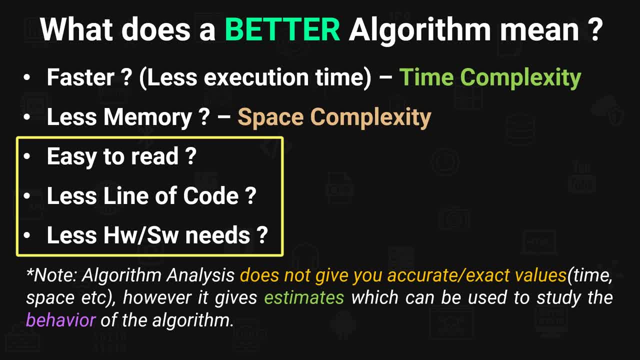 less lines of code. So let's say, an algorithm A is doing the same thing in 10 lines, whereas my algorithm is doing in 20 lines, So maybe your algorithm is better. Another criteria can be is your algorithm requiring less memory? 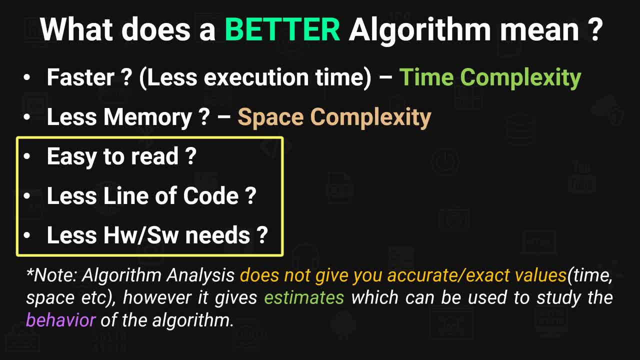 Yes, Hardware and software requirements. So nowadays you must have seen that some programs only run on windows 10.. They are not running on windows seven. So you can see that some programs also have software requirements. So it's not just hardware requirements. So 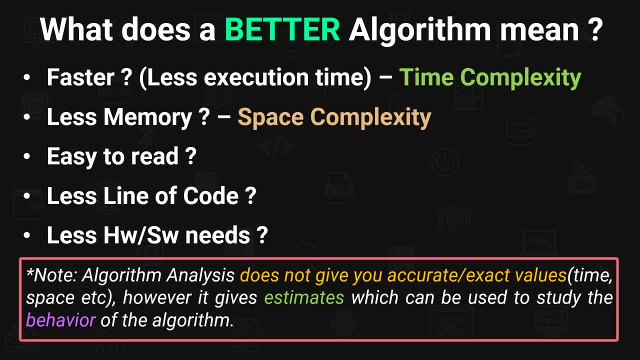 as you can see, there are so many different things and that's why you can see there is a note over here. Algorithm analysis does not give you accurate or exact values. However, it gives us estimate which can be used to study the behavior of the algorithm. Now. 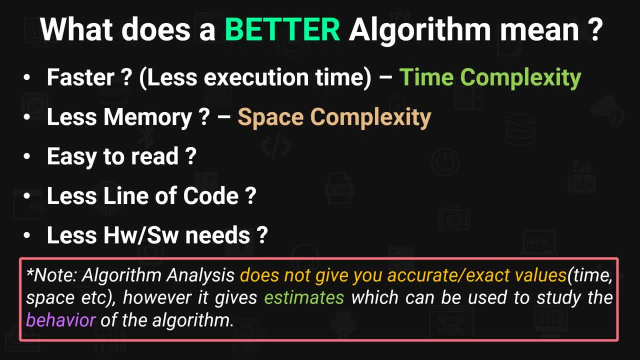 because there are so many different criteria, there are so many different conditions. So you cannot pinpoint and see that my algorithm is going to run in exact two seconds because, let's say, you and I have the exact same laptop, exact same specifications, all the hardware. 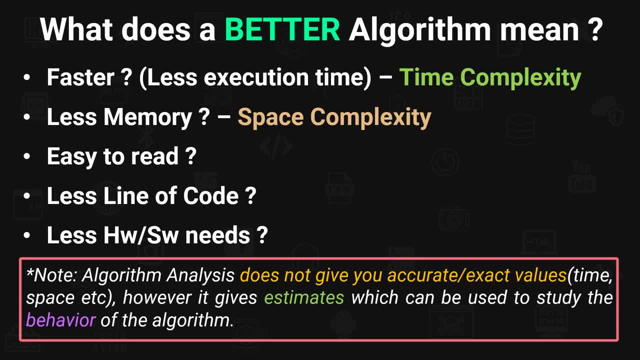 and software specifications are exactly same. However, on your system, along with your algorithm, you have 10 programs, but on my system I don't have any other programs. So CPU is directly only going to focus on my program and my program will execute faster. So you can see just by. 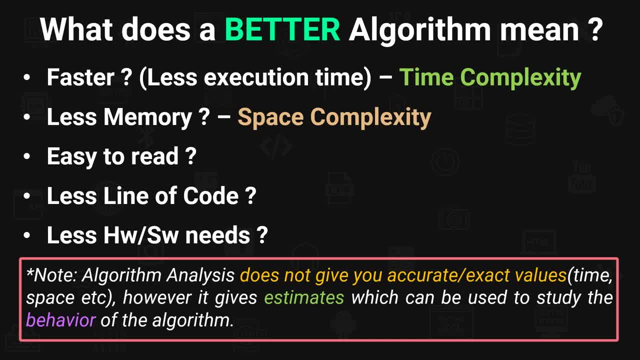 addition of extra programs in your system. even the everything else was same. still my algorithm ran faster, right? So you can see there are so many different criteria. So that's why algorithm analysis does not give you accurate values. Now this takes us to the next big question. that is then: what is asymptotic? 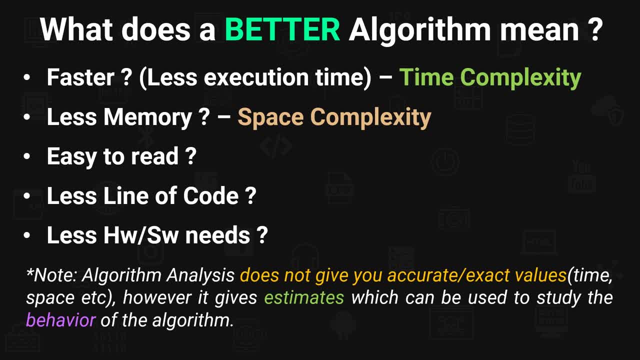 algorithm analysis. Now we've understood overall what is algorithm analysis: basically studying the time and space complexity, how much time the algorithm takes, how much space the algorithm takes. So we have a category of analysis which is known as asymptotic analysis. So 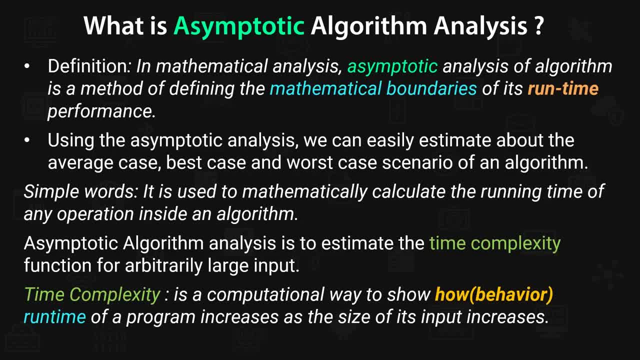 let's take a look at that. So when you're studying data structures and time and space complexity and this algorithm analysis, you must have come across this asymptotic algorithm analysis concept, focusing more on asymptotic word. Now, the definition can be as follows: 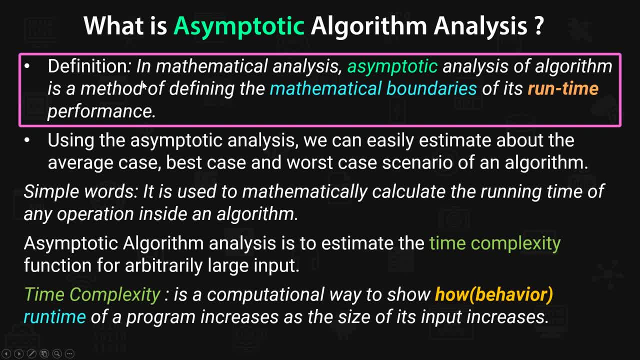 So in mathematical analysis, asymptotic analysis of an algorithm is a method of defining the mathematical boundaries of its runtime performance. So quite a lot of big, big words are used over here, but over here you can see in simple words what it is doing is it's trying to 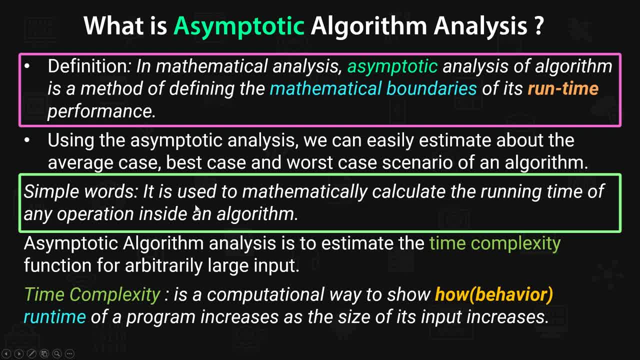 do is it is used to mathematically calculate the running time of any operation inside an algorithm. That's the easy way to put it. So what happens is, when you're measuring the performance, you want some numbers right. So ultimately, it is basically mathematics. 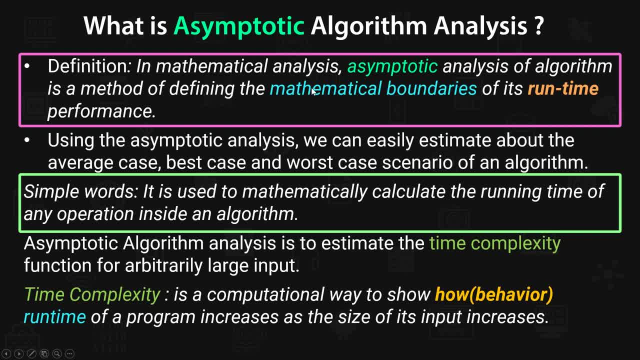 So what we're doing is we're using this technique to define the mathematical boundaries. When I say boundaries, it means the upper and lower limit of an algorithm, of its runtime performance. So runtime is basically the time required for an algorithm to execute. Now you can see that asymptotic algorithm analysis is more dealing with the time complexity. 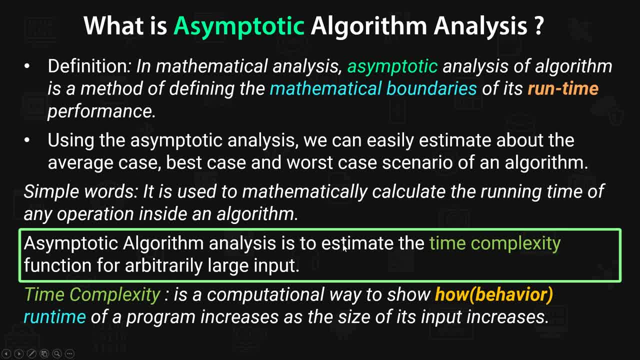 So you can see point over your asymptotic algorithm analysis is used to estimate the time complexity function for arbitrarily large input. So when you're talking about algorithm, if everything else is kept constant- when I say everything else, it means the PC, the hardware, the 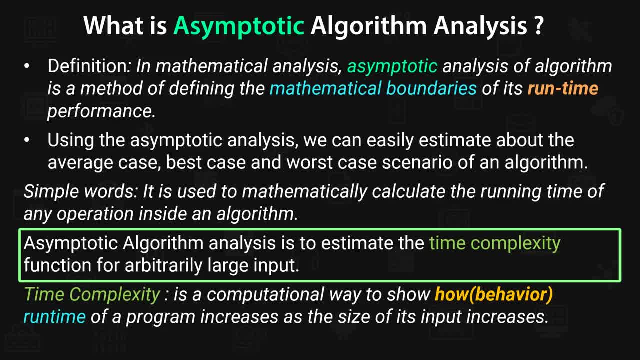 the CPU, the Ram, whatever hardware things you're using, whatever software you're using, if all those things are constant, which in usual cases are constant in an environment- the only thing that changes is the size of the input, which means how many number of. 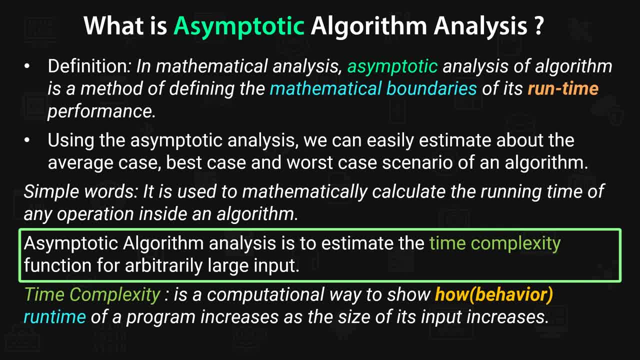 steps are there in the algorithm, So that depends upon what input you give to that algorithm, right? And you'll see that if you're confused, you'll see this in the very next slide or as you move out in this video. So hold tight, don't get confused. So essentially we are. 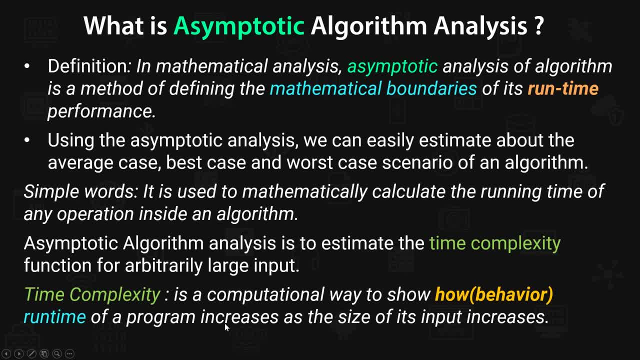 studying the behavior of an algorithm for a large input, to study the mathematical boundaries, For example. we are studying how an algorithm performs when it has thousand steps or 10,000 steps, Because you want to study its boundaries. Okay, So, using the asymptotic analysis, we 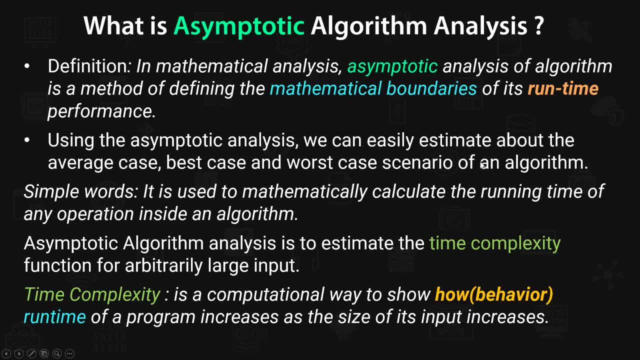 can easily estimate about the average case, best case and worst case scenarios of an algorithm. So when I'm talking about average, best and worst case, it means the time. Okay, So the best time in which the algorithm can execute. that is, how fast can an algorithm execute? 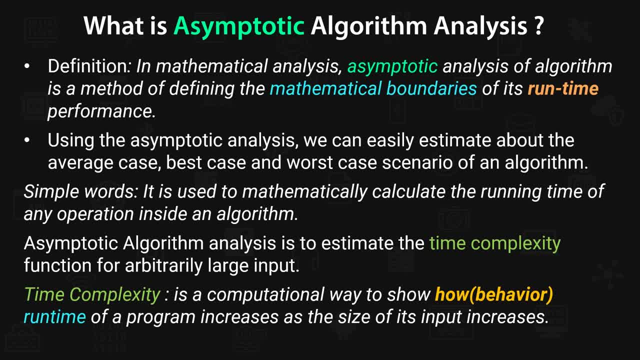 How slow can an algorithm execute and what is the average case? Okay, So ultimately, time complexity is a computational way, Basically a mathematical way, to show how runtime of program increase as the size of the input increases. So you've come across time complexity quite a lot in this entire. 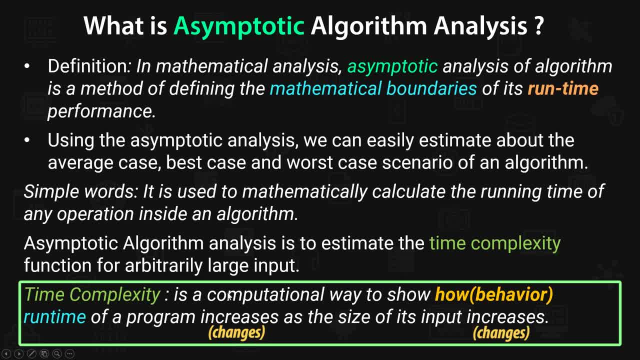 slideshow. So most basic definition is: it is a computational way to show how the runtime of a program increases as the size of the input increases. So how means the behavior? So let's say there are 10 steps in a algorithm. for 10 steps, How many seconds or micro seconds? 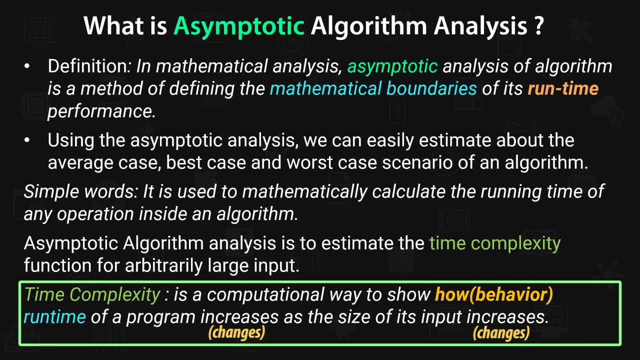 is it taking? Is the algorithm taking io, If I double that steps, if I make 20 steps? is it increasing linearly or is it increasing exponentially, right? So that is what we are trying to find out, That is what asymptotic. 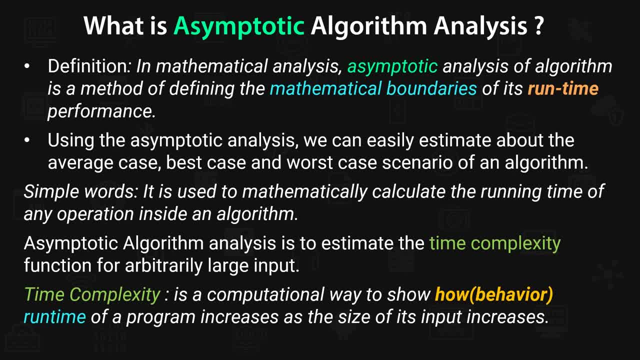 algorithm analysis is helping us do. Now, I know this was a lot of theory, right, So let's actually take some example, because then we can easily jump on to the next big topic, that is, big O notation. Okay, so, as you can see on the screen, I have switched to our digital blackboard and now we 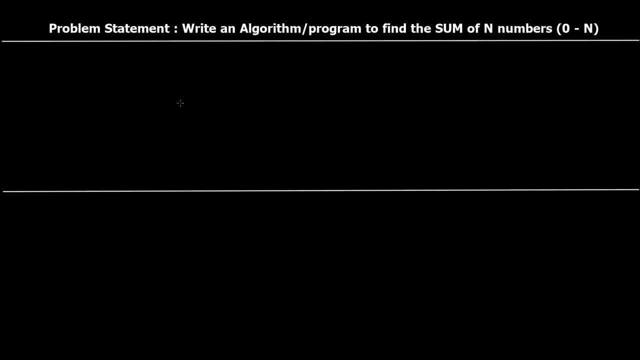 are actually going to take a practical example to understand asymptotic algorithm analysis and understand what is big O notation. Okay, so what is the problem statement over here? Now we've been given a problem statement over here which is write a algorithm slash program, which we are kind of. 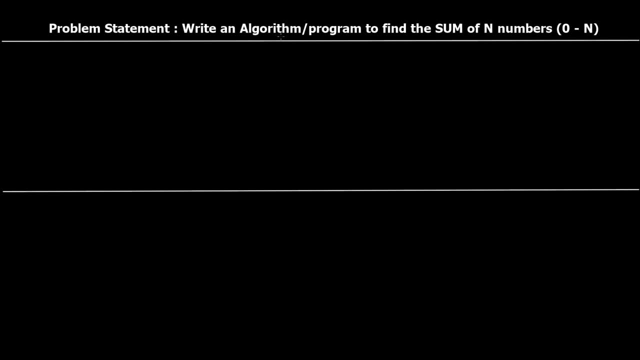 assuming one and the same thing. So, essentially, what is algorithm? It is just step-by-step process and when we convert that algorithm into programming code, we call it program. right, So we are assuming it as one and the same thing. So what we have to do is we have to write an algorithm or program. 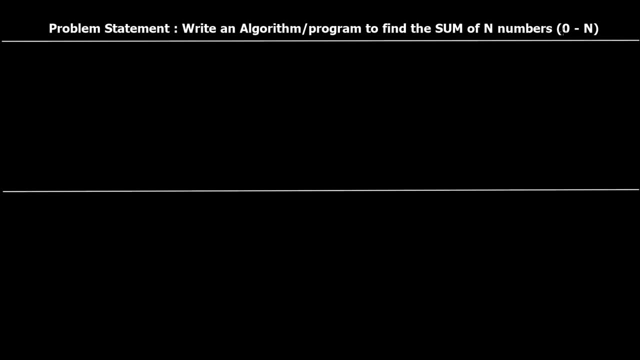 to find the sum of n numbers. So n numbers would be ranging from 0 to n, and this n is supposed to be accepted from the user. So we will take n from the user. Let's say user enters 3. So it would be 1 plus 2. 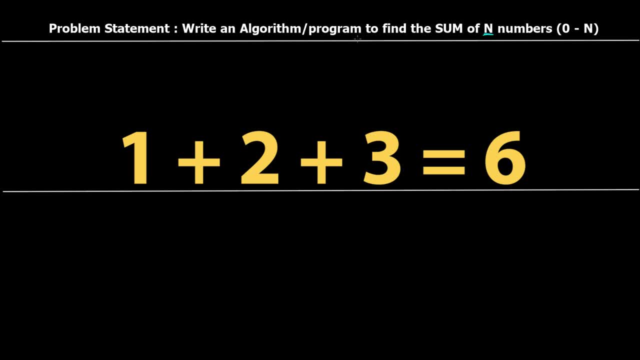 plus 3, and the total would be 6.. So we have to print out 6.. Okay, so that is the problem statement. If the user enters 5, it would be 1 plus 2 plus 3 plus 4 plus 5, and then we have to. 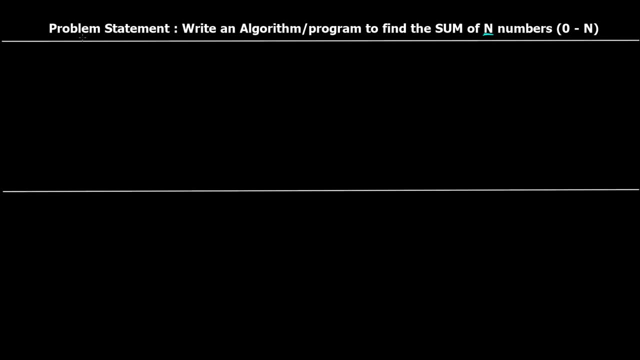 print out the total. So I hope you've understood the problem statement. It's basic. Now, to solve this problem statement, we have multiple approaches. If you didn't know that, you can Google it out, But let me just show it to you right now. 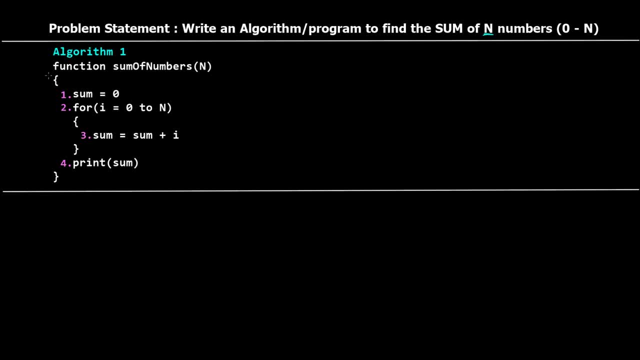 So here's algorithm number 1 or method number 1.. You create a function and this is not exactly any kind of programming code. It is kind of like a pseudo code, but it's pretty understandable. You're creating a function, You're naming the function as sum of numbers and you're 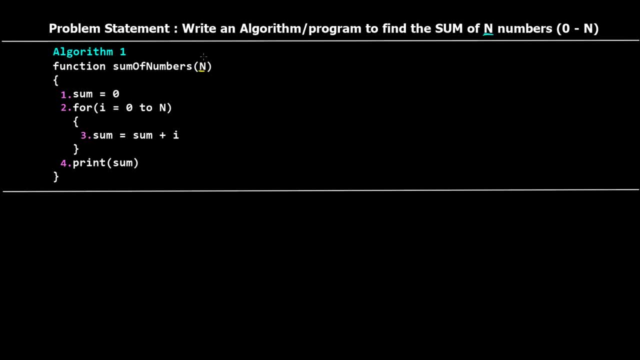 passing arguments as n. So this is something that the user will enter. First step is you declare a variable sum, assign 0 to it. Second step is a for loop. Now you run a loop from 0 to n, Or you can say 1 to n also, And then you say: sum is equal to sum plus i And all the values stored. 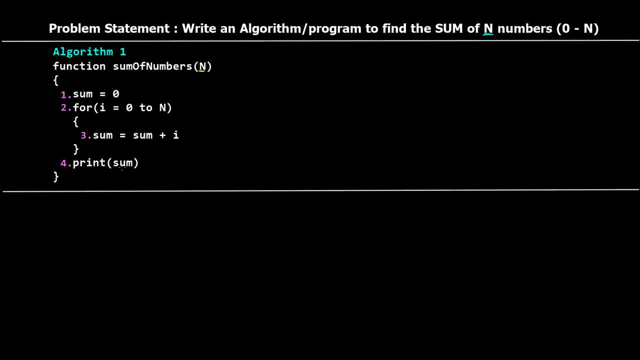 in the sum variable itself And ultimately, at step number 4, you print the sum. So if you enter 3, your for loop will run from 0 to 3.. That is 4 times. Okay. you can also run it from 1 to 3.. 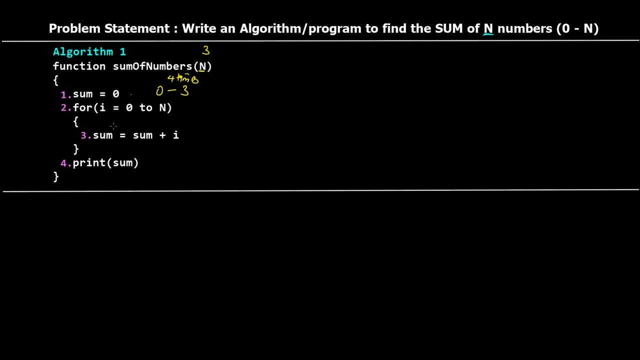 It would run one time less, but that's okay. What will happen? Initially, sum would be 0. So it would be 0 plus i is 0 for the first time, So 0 will be stored. Next time it would be sum which is 0 plus i will become 1.. 0 plus 1.. So 1 will be stored over here. 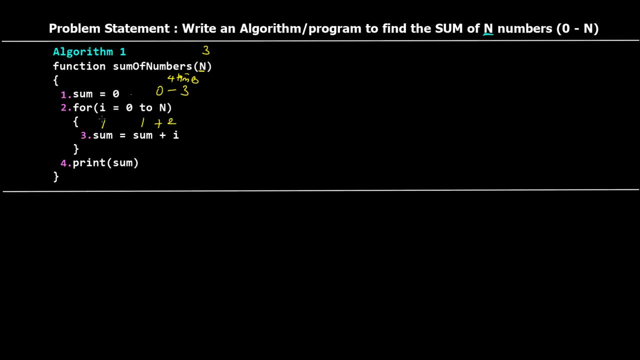 Next iteration it would be 1 plus i will now become 2.. So 3 will be stored over here. For the next iteration, 0 will become 3.. So it will be 3 plus 3.. So 6 will be stored over here. 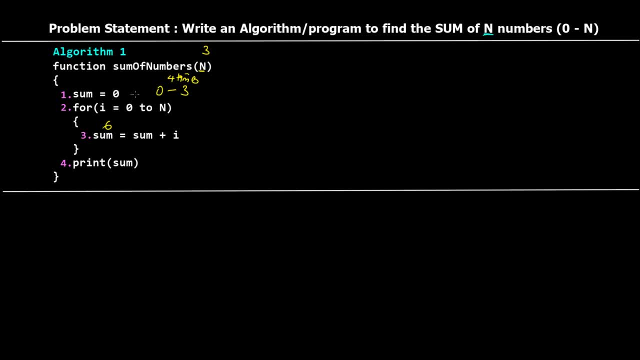 And now the loop will exit, because i will become 4.. We are only interested in running from 0 to 3.. So after this, we will print the value of 6.. So basic enough. Now, what we'll do is we'll. 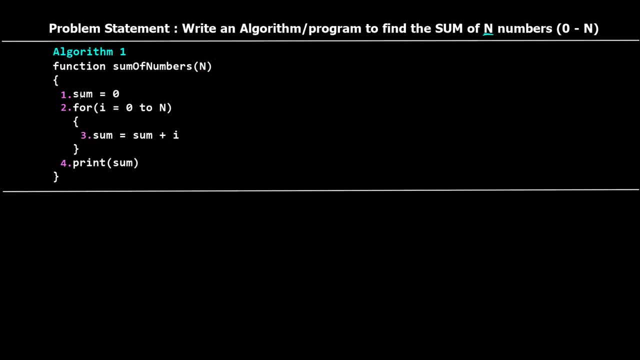 assign a function to the loop. So we'll assign a function to the loop. So we'll assign a function to the loop. We'll assign some time for individual instructions. So you can see, this algorithm is nothing but a step-by-step instructions. So we have instruction number 1,, 2,, 3, and 4.. So let's assume this first. 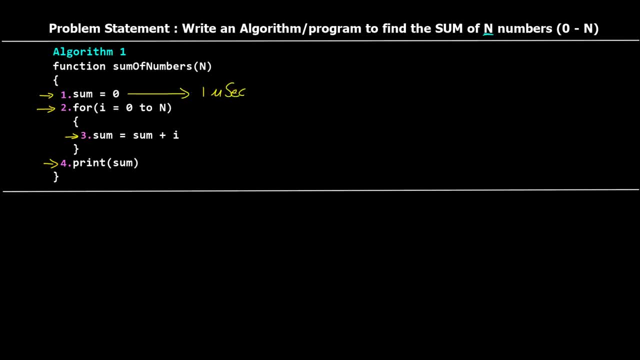 instruction is taking 1 microsecond. Now we are just making some assumptions. Obviously, every instruction is going to take some time, but it is not going to be 1 microsecond. I'm just making an assumption. Okay, But obviously every instruction is going to take some time. 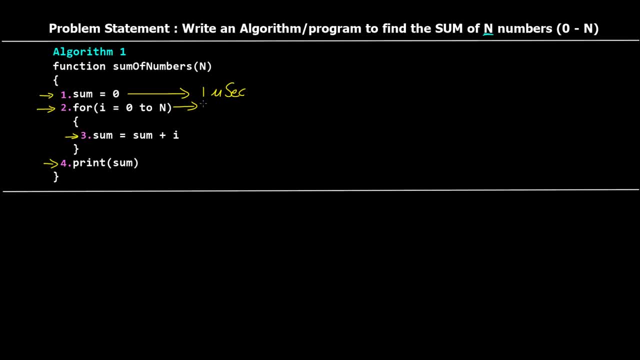 Let's say, the second instruction is the initial. It will also take some time. We'll again assume it as 1 microsecond. Now, this third step is totally dependent upon this n value, right? Because whatever value we enter over here, let's say we: 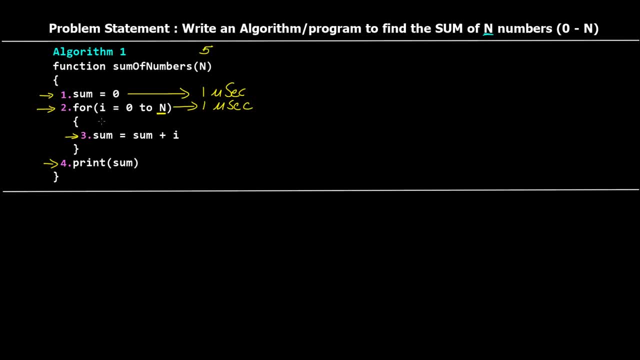 enter 5.. So this for loop will run for 5 times. If it starts from 1, let's assume it is starting from 1.. It will execute for 5 times, from 1 to 5.. If we enter 6, it will run for 6 times. So for this, 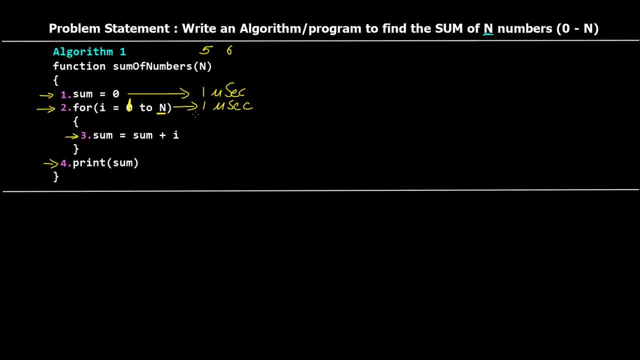 let's say, one step, running it for one iteration takes 1 second. So for n iterations it will take n microseconds, right? And then again, this last step is just printing the sum out. Let's assume it takes 1 microseconds. So after assuming all these values, we can conclude that the time 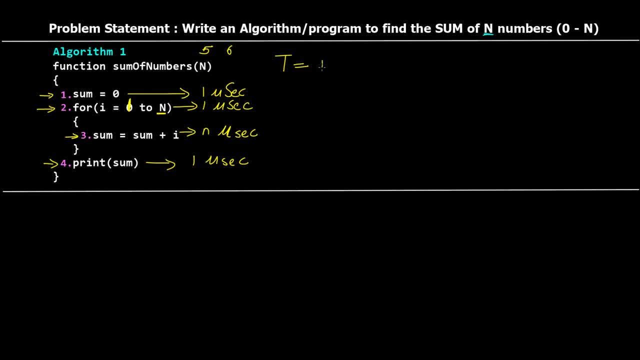 required by this algorithm is something like n plus 1,, 2, and 3, 3 microseconds, right, And this 3 microseconds is 1 microseconds. So we can conclude that the time required by this algorithm is always going to be constant. Only this n is going to be a variable. So this is that n. I'll do a. 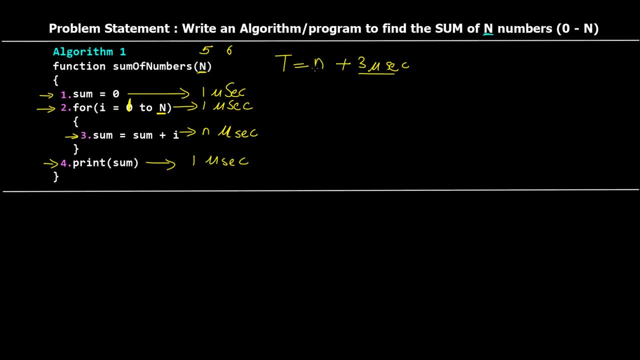 small n for time and capital N for size. So this n will keep on changing. So, depending upon this n, the time will change, right? So you can make a clear observation over here and you can make a graph of this. So how will the graph look like? So, as you can see over here, this is how the graph 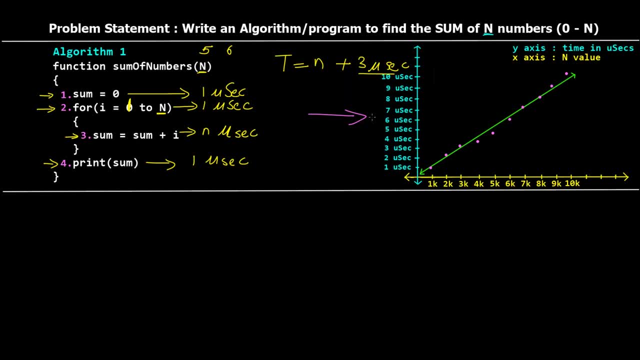 would look like for this algorithm 1.. So what is this graph? So on this axis we have the n value, which is whatever value entered by the user. So 1k is basically 1000, okay, So I'm assuming it for large numbers If the user enters 1000 over here. 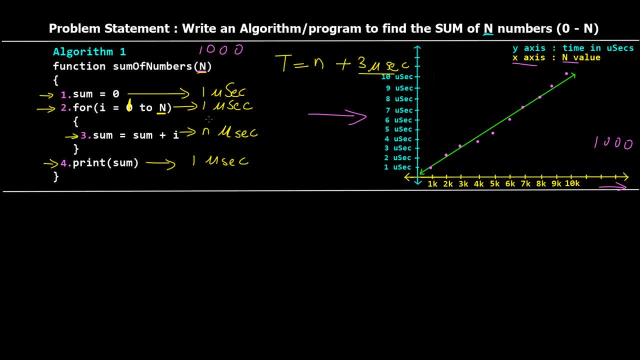 this inner step will run for 1000 times, right? So this would be 1000 seconds. So it would be 1000 plus 3 microseconds, So ultimately it would be 1003 microseconds. Now again, I'm telling these: 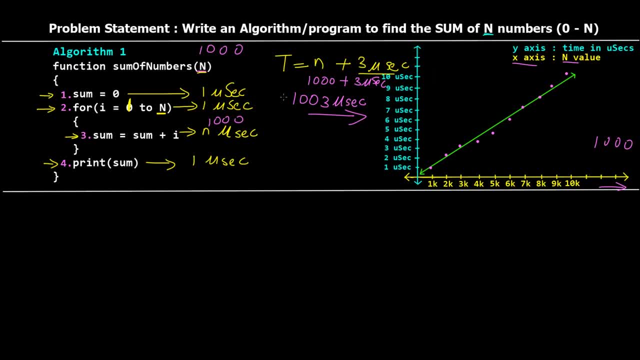 are just estimations. These are not actual values, but this is something that would happen, right, In reality also, something like this only will happen. So over here you can see that for 1k value of n, this y-axis is basically the time in microseconds. okay, So this is in microseconds. 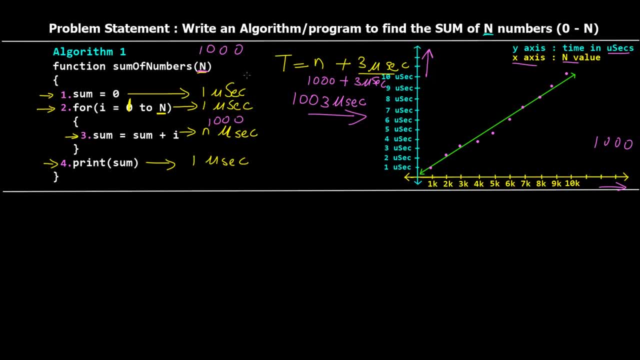 For 1k it is taking 1 microsecond. So we are assuming it is taking 1 microsecond when you enter 1000.. When you enter 2000 as sum of 2000 numbers, it is approximately taking 2 microseconds. 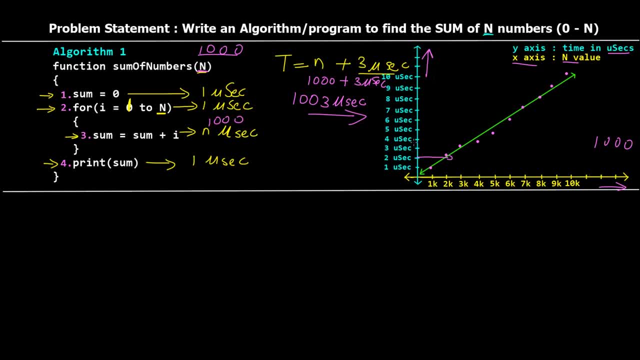 It is a little above 2 microseconds because obviously n is representing the exact values. We've just talked about that and you cannot never estimate exact values For 3k. if you enter 3000, that is sum of 3000 numbers. it is somewhere taking. 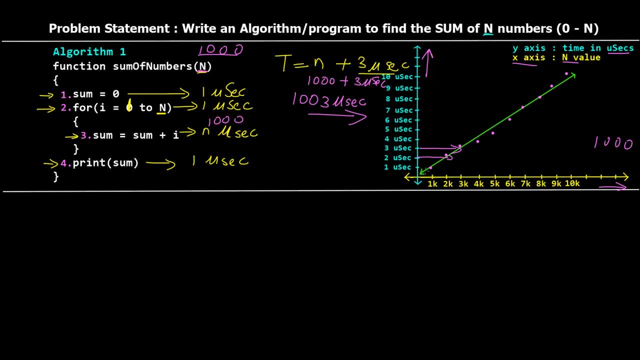 3 microseconds And you can see that this trend is going in this direction. So this basically is called a linear behavior. So when I say linear behavior, it means that as the size of the input increases, obviously this n is representing the size of the input, because n is basically. 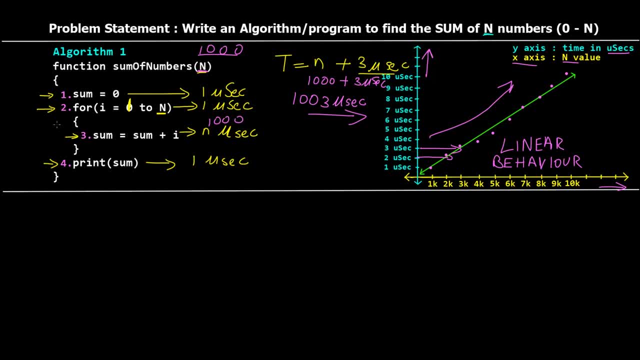 corresponding to the number of times this for loop will run right. So if n is 10, this for loop will run 10 times. So we have 10 steps. So that is basically the size of the input. So as that is, 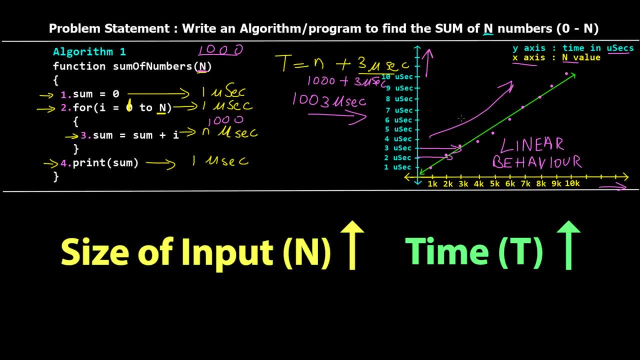 increasing. you can see the time taken by this algorithm to run is also increasing And it is increasing in a linear way. So you can see this is a straight line which is going up and up as the size of n increases. So this is a linear way. So for this algorithm, the time complexity you can 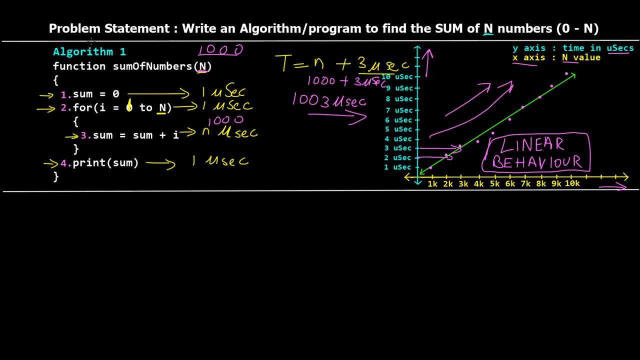 see is increasing. So that's why I've said linear. let's take the same problem statement And let's see one more algorithm for the same problem statement. Okay, so, as you can see on the screen, this is algorithm number two and it is surprisingly very small. So you're wondering, okay, is it? 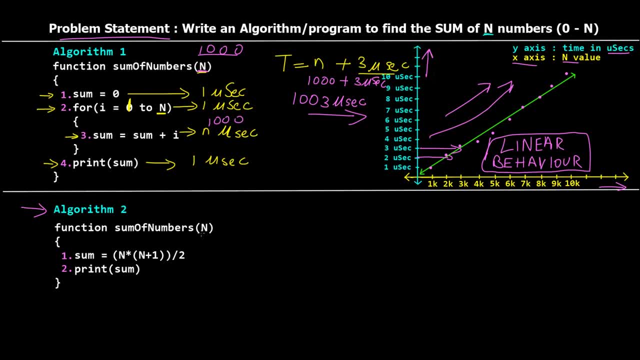 doing the same thing. So again the same function: sum of numbers. it is taking n from the user. However, in step number one, we are declaring a variable sum and we are saying it is equal to n star, n plus one, the whole divided by two. So where did I get this? Now, this is: 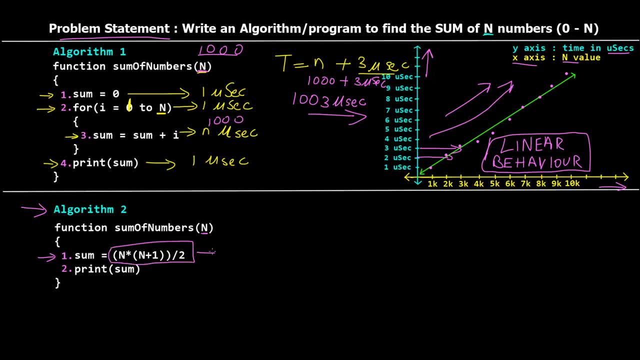 a mathematical formula for calculating sum of n numbers. So for those who don't know, it's a mathematical formula. you can google it out And that is the reason why you have mathematics in computer science and information technology oriented domains also. So whenever you're going out with 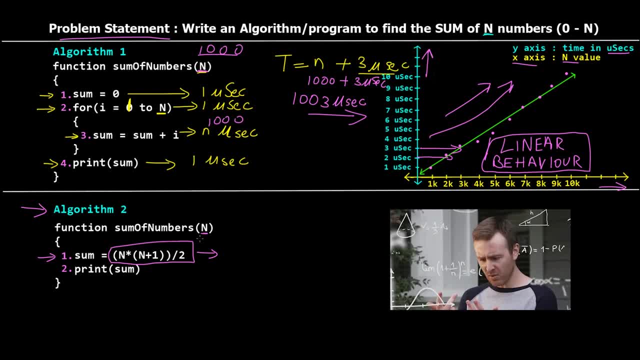 a course of IT or computer science. students generally complain about: why do we have mathematics? it is for this reason. Okay, so you can see directly: at this step itself we are directly getting the sum and at step number two we are just printing it. So again, if the user enters, 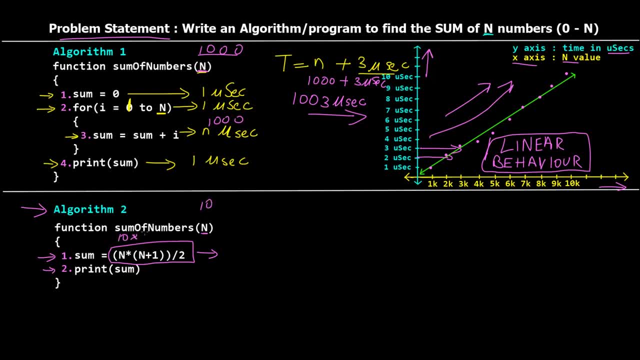 10, we simply substitute 10 over here, 10 into again 10 plus one, the whole divided by two. if the user enters 100, we simply have to substitute 100.. So you can see there is no for loop or there is no. 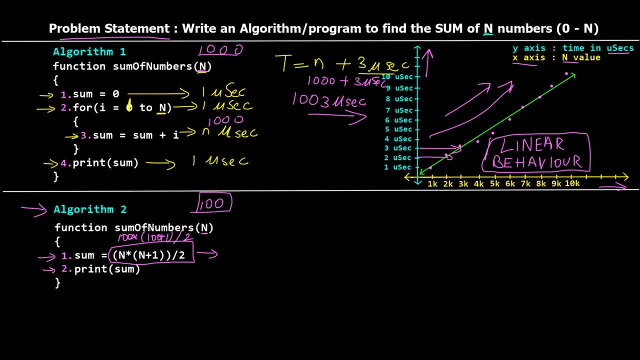 multiple iterations. we are simply entering this value inside this formula. It's that easy. So let's assume this takes two microseconds. okay, and this step takes three microseconds. So no matter what input you provide, if n is 100, or n is 1000, or 10,000, or one lakh or whatever the value this step is only going to take around. 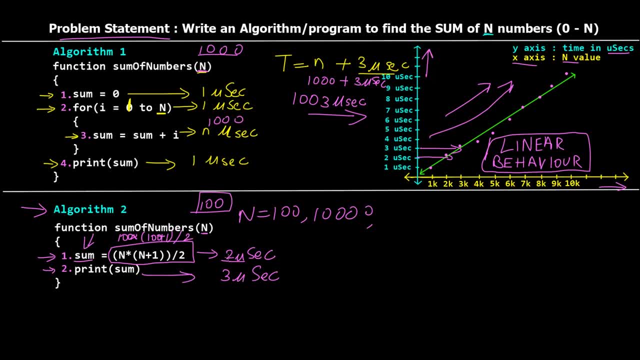 two microseconds. I'm not saying it is going to take exactly two microseconds, but it won't take a lot of time. right, it will take two seconds or three seconds or something like that. So you can see, even when the n number is increasing, the total time over. here you can say that T is equal. 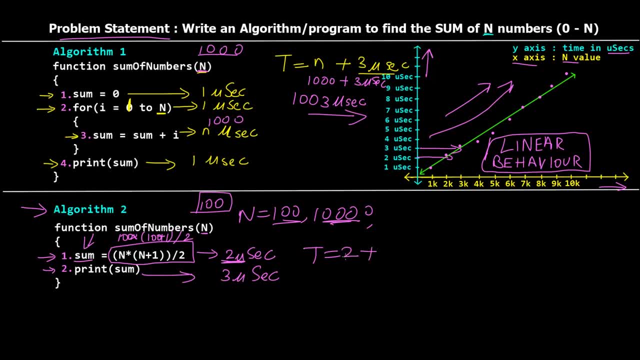 to this two seconds, or two microseconds, plus this three microseconds, Or we can just consider it as 1 microsecond, because printing does not take a lot of time. so 2 plus 1 is 3 microsecond. so no matter what the value of n, your algorithm is taking 3 microseconds, which is constant. so this is some. 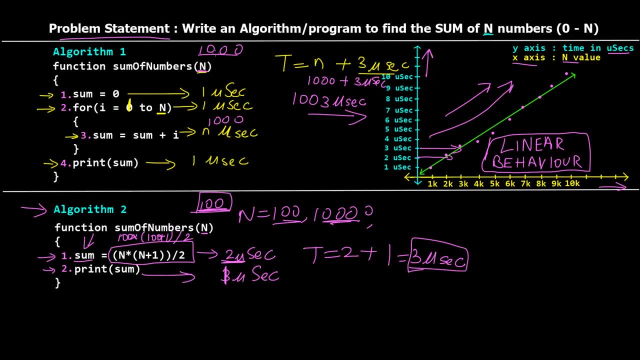 weird behavior. right, this is not the same behavior as algorithm 1. in algorithm 1, as the size of the n value was increasing. as this n value is increasing, the time is also increasing. however, here, no matter what the value you enter, your time is approximately going to be the same. so how does 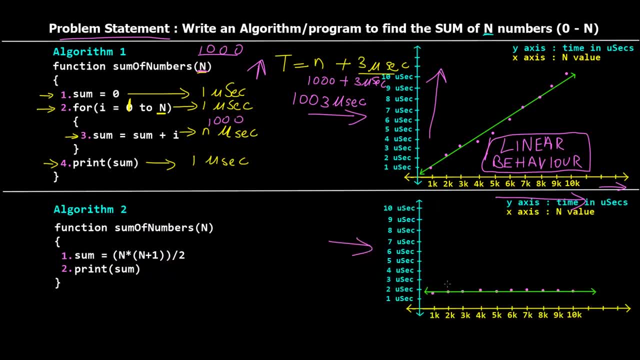 the graph of this algorithm look like. so this is how the graph for this algorithm 2 looks like. now you can see it is a straight line. however, it is not an increasing line. so no matter what the size of n. so you can see n is over here 1k, so n is 1000. when n is 1000, it is taking 2 microseconds. 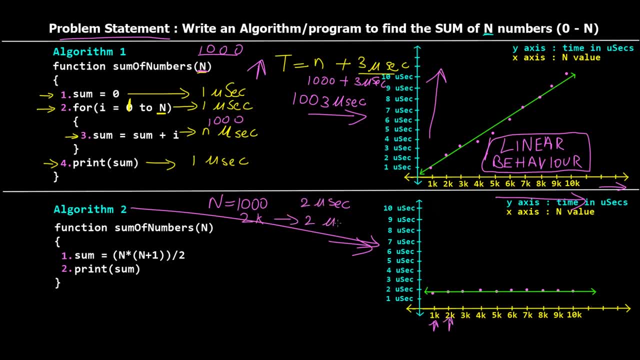 when n is 2k, it is still taking 2 microseconds. you, when n is 3k, it is still taking 2 microseconds. when n is 4k, it is taking slightly greater than 2 microseconds because obviously it is not going to be accurate values, but you can see overall the 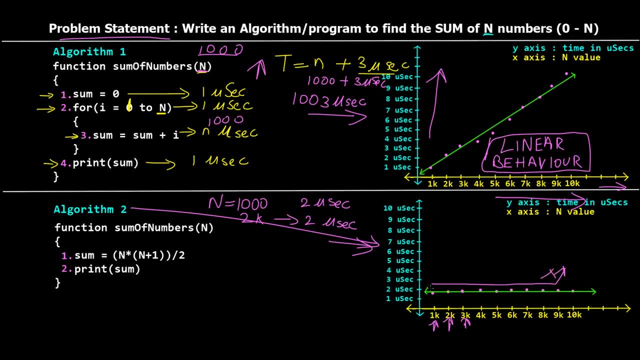 time is not increasing. it is not increasing, it is constant. so this behavior is known as constant time behavior. okay, so when you are doing analysis of algorithm 1, we are getting linear behavior. but for the same problem statement, we are typing or writing algorithm 2 and it is giving us 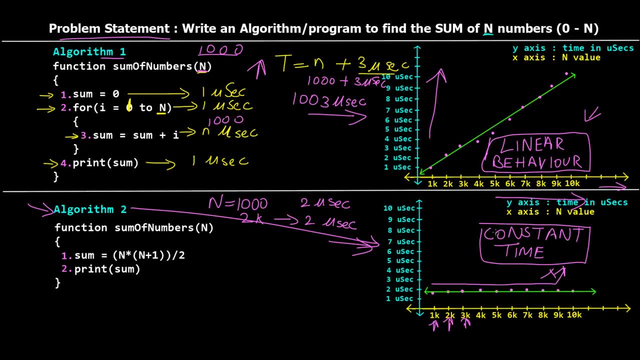 constant time behavior. now, just by observing it, you can say that obviously, algorithm 2 is much more efficient than algorithm 1. now, if you are still confused, or if you are still wondering, does it actually give the same value? let's actually jump to the code. let's actually open. 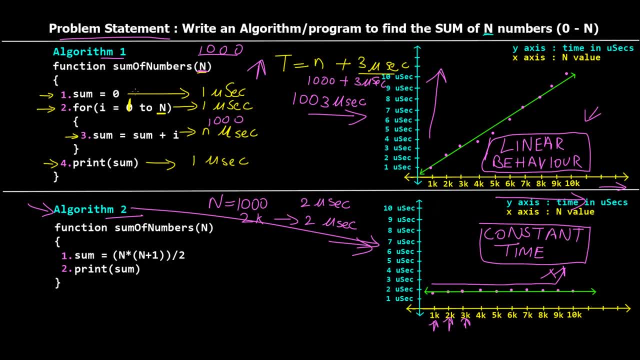 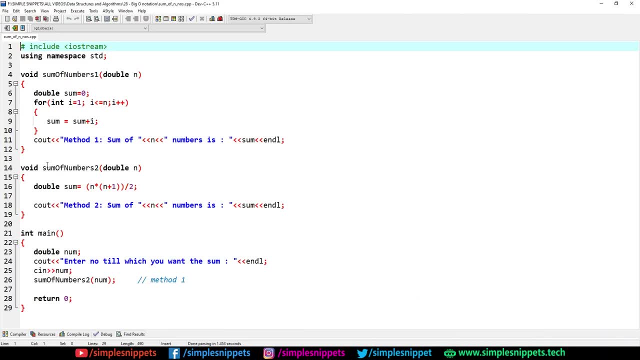 up dev c++ and type a c++ program to execute these two algorithms, and i will show you live what happens. okay, okay, so, as you can see on the screen, i have already typed in the code because the algorithm was pretty basic. so this is you: the hash include iostream and the basic boilerplate that you have to type when you are typing. 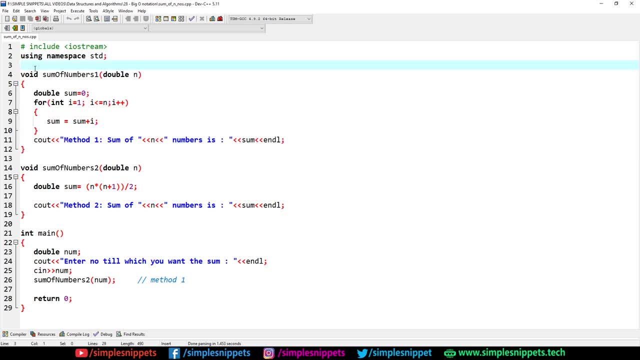 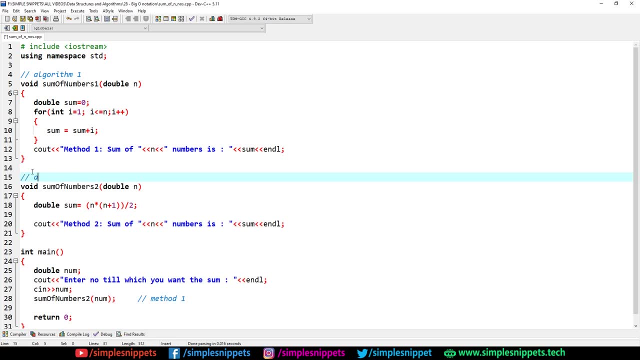 c++ programs. so this is function number one. or you can say this is algorithm 1, let me just type it. and this is algorithm 2. so i have typed in two different functions, which are those two different algorithms that we just saw. if you want, i'll put it on the right. 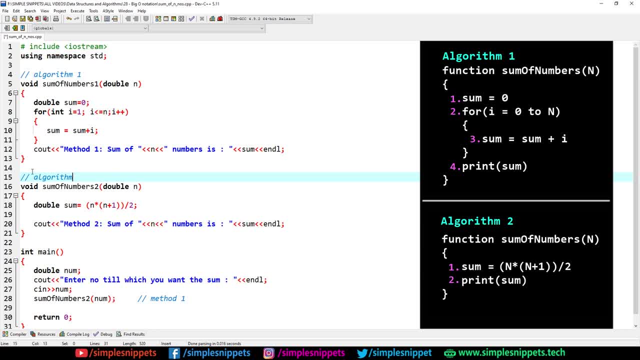 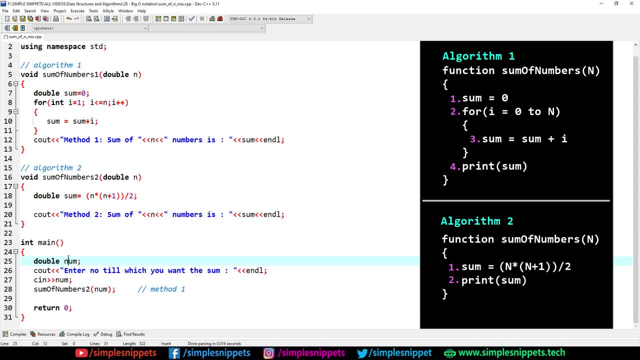 hand side on the screen you can see and correlate with the algorithm steps as well as the program steps. they are the same. this is algorithm 2 and in the int main you can see i'm just declaring a double variable which is double num. the reason why i'm declaring it as a double is because we are 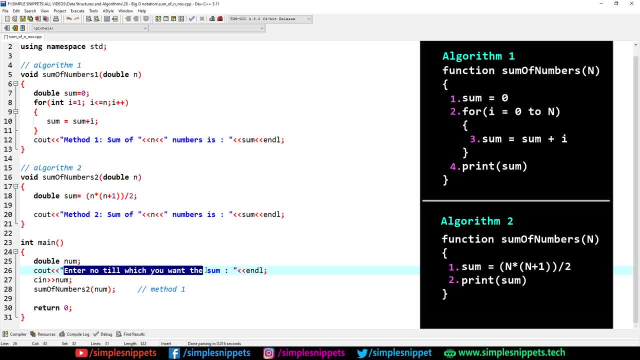 going to enter a large number and then we are asking the user to enter that number, we're taking it from the user c in and we are passing it into either of these two functions. so function number one is sum of numbers one. function number two is sum of numbers two. basically algorithm one. 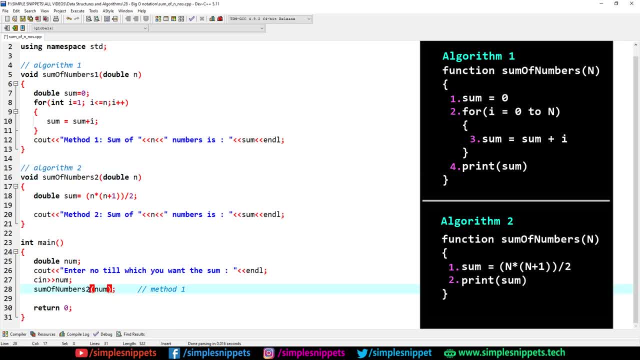 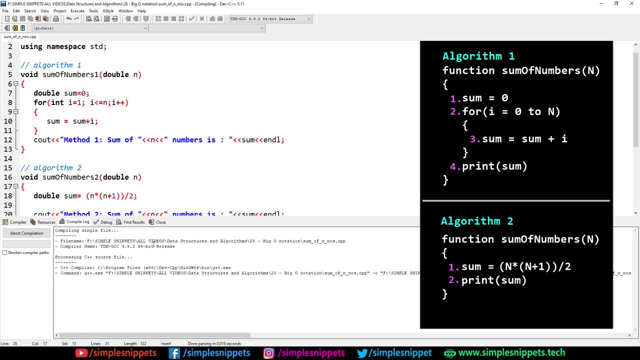 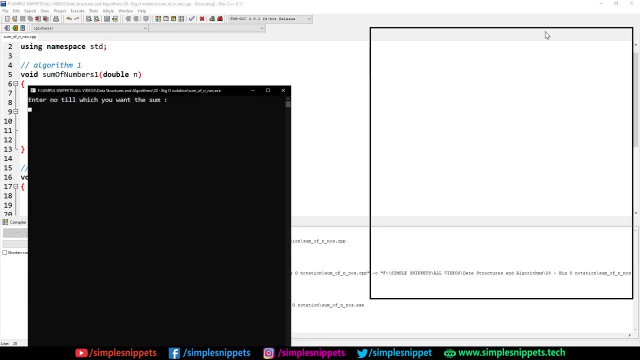 and algorithm two: okay. so let's first call algorithm one: okay. sum of numbers one. save this, go to execute and first let's just compile it. it will take some time. this is not the execution time, by the way. now you go to execute and let's say compile and run. okay. so as you can, 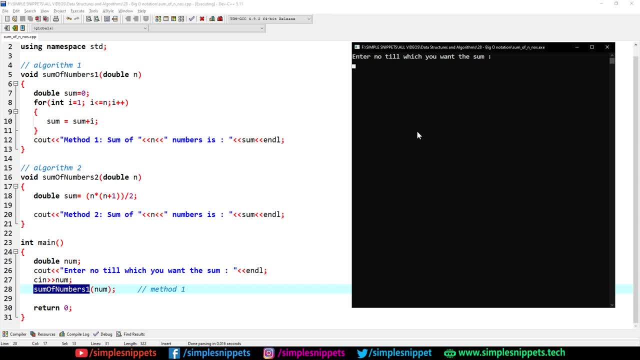 see on the screen, our program ran successfully because obviously I've already written it properly. if you want this entire code, I will share in the video description, but I would recommend that you type it. but now it is asking: enter a number till which you want to find. 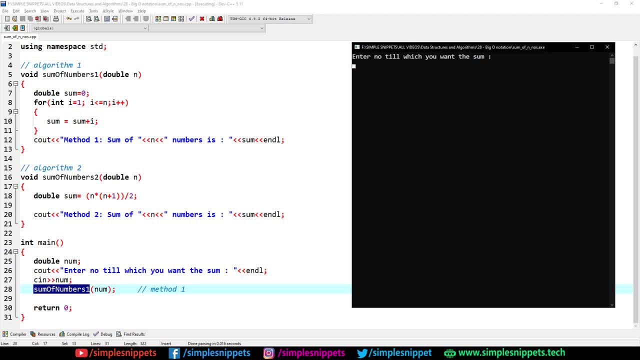 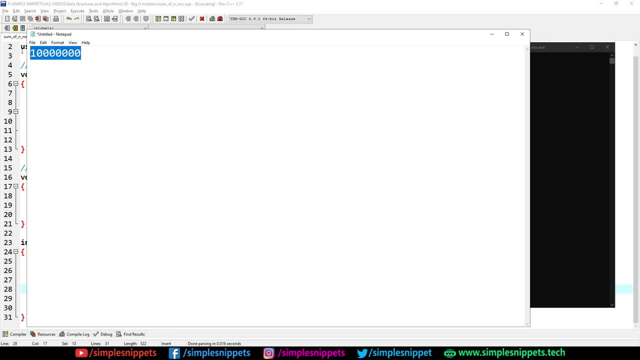 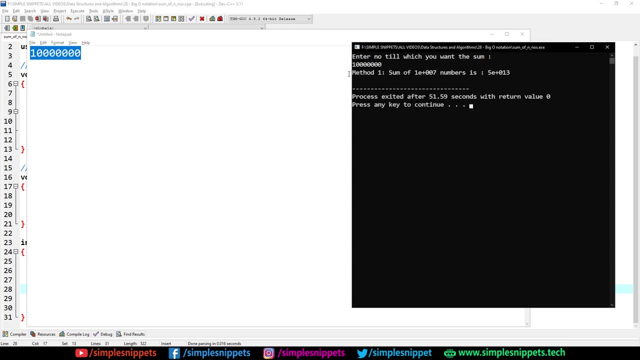 the sum. so let's enter a very large number. let me go to the notepad and type in some large number. this is 100,000,1000, 10000,, 10000 crore, right? so this is one crore. let's copy this and paste it over here. if I hit enter, we are directly getting the sum. very 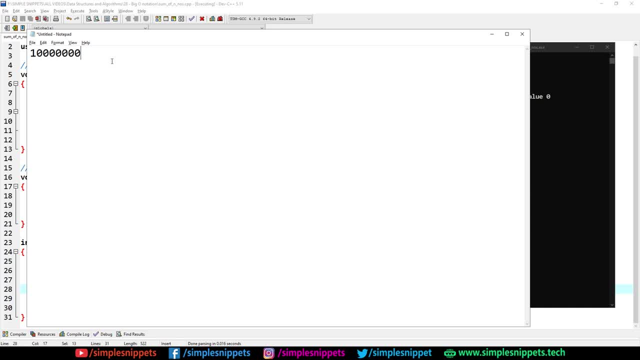 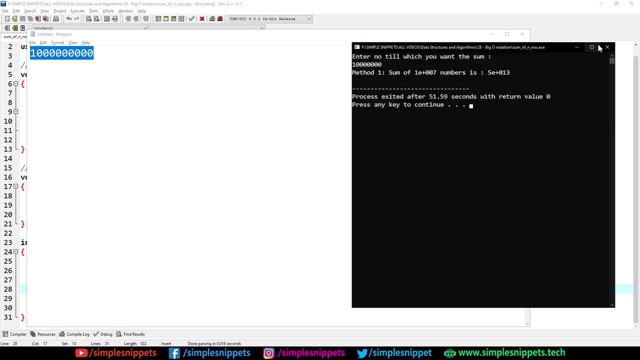 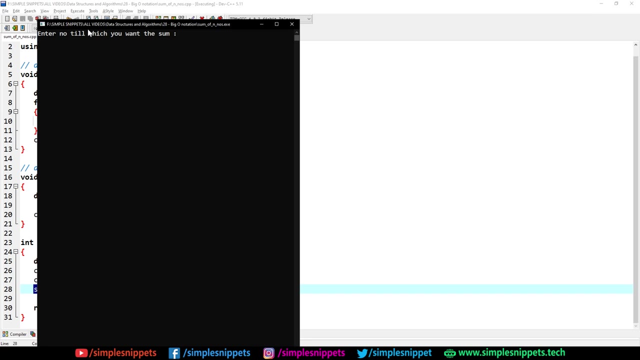 easily because we still need to put a very large number. okay, So this is one crore. let's enter ten crore, hundred crores. let's copy this and let's try to again actually execute this and enter a large number. Okay, 100 crores. so if i hit enter and hit enter, you can see it is taking some time: one, two, three, four. 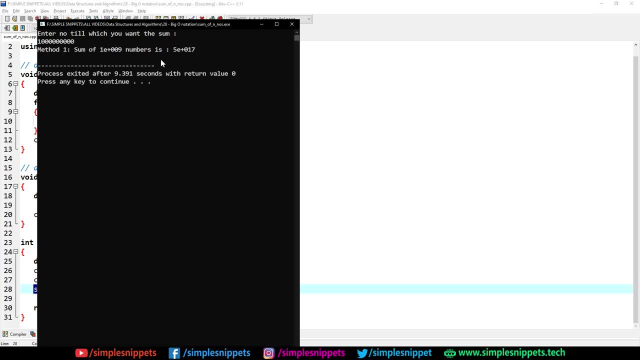 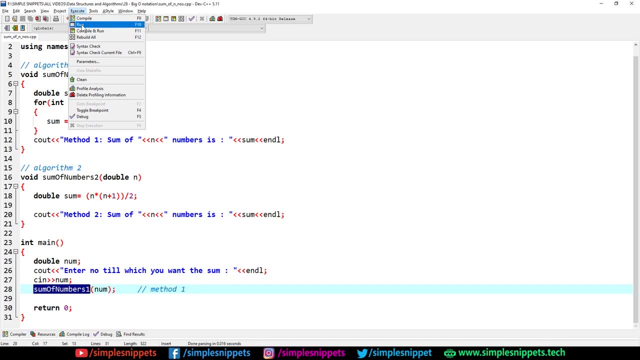 five, six, seven and you can see it took seven seconds to execute and i was literally counting it in front of you guys. so let's just do it again: go to compile to go to execute and run. let me just put it out properly over here. so i'm putting 100 crores as the number because 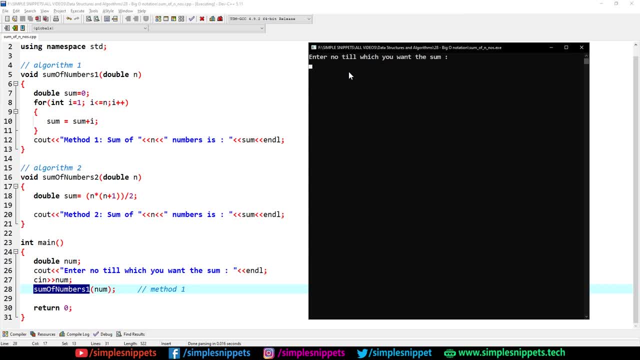 it is a very large number and it should take some large amount of time paste. so this is 10 crores. if i hit enter and start the countdown, i'm gonna hit enter and start the countdown. one, two, three, four, five, six, seven, eight, and you can see it took around eight seconds. so this is. 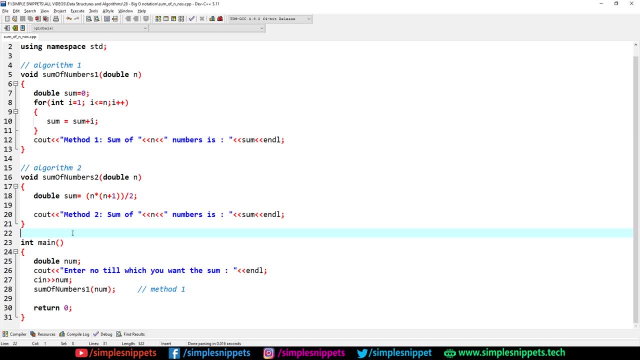 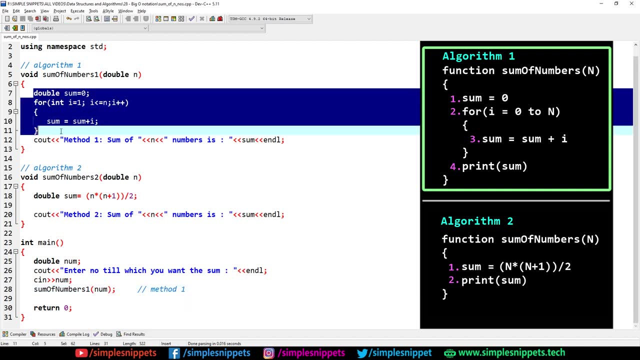 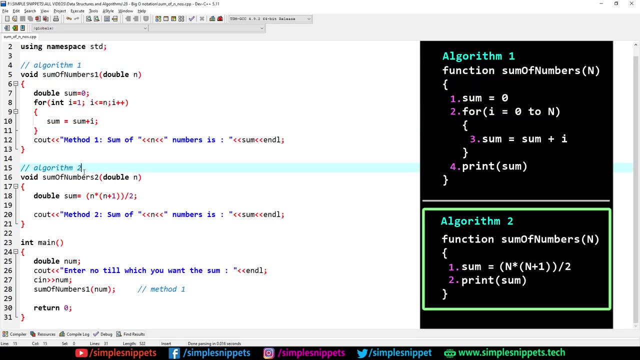 100 crores. okay, let's close this. now let's come to our code. and so this was algorithm one, which was linear complexity, which was when the time was increasing with the increased amount of size of the input. now, what we will do is we will run algorithm two, which was a constant time behavior algorithm, so it was like no matter. 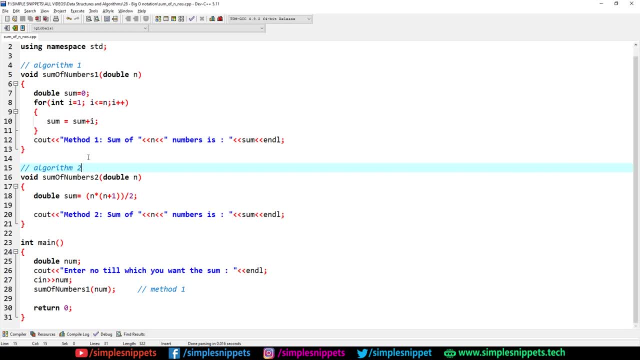 what the size you give. the algorithm was running in that exact time, okay, so i'm gonna make that change over. here we are calling sum one, sum of numbers one, which was algorithm one, so i'm gonna make it to sum of numbers two. okay, save this first, compile it. okay, make sure you compile it, because 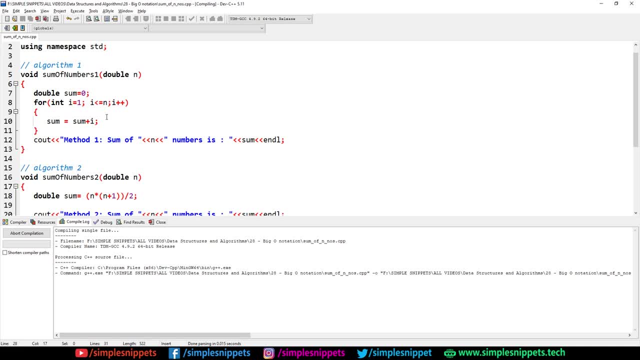 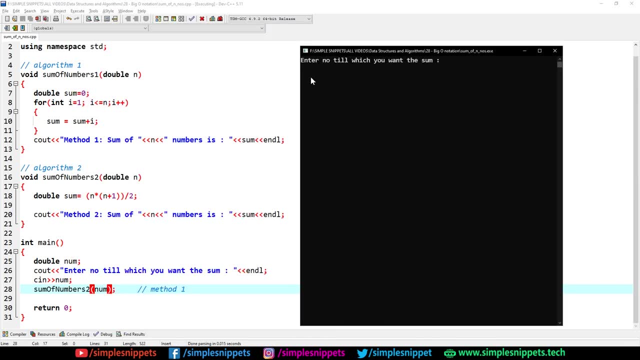 otherwise the previous code will run. so i'm gonna hit compile- it's compiled successfully. close this. i'm gonna say run. so now we are basically running method number two, so we'll also see the output in method number two. this output will be printed. earlier it was method number one. let's come back. 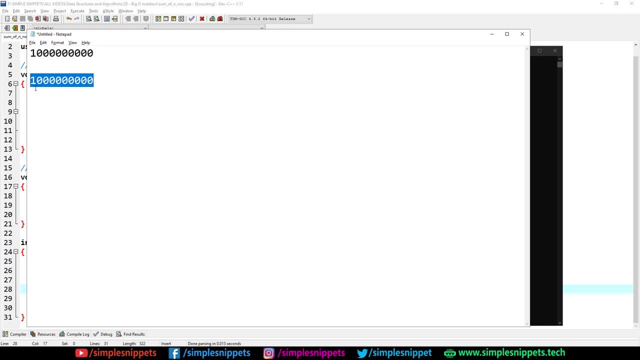 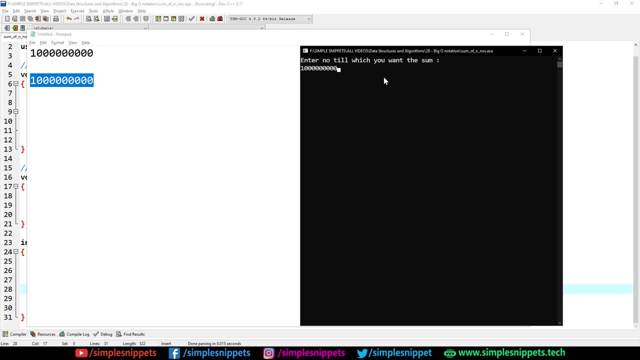 to this notepad. let's copy this number, which is more than 100 crores copy. come over here, just paste it. if i hit enter and start the countdown, actually it will give us the answer immediately. it will not take eight seconds. it will not take 10 seconds because it is constant time. 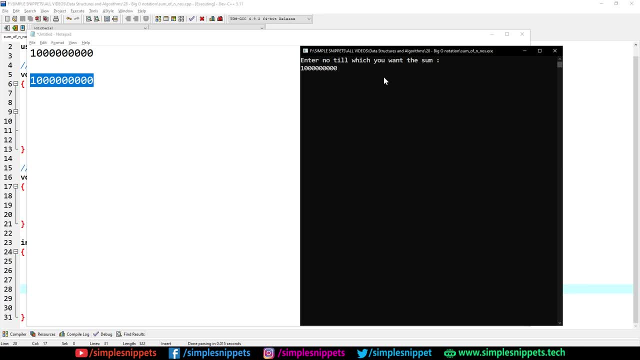 it will not get affected by the size of the input. let me just show you like i'm now hitting enter and there you go directly. i got the answer. you can see method two: sum of this large value is represented as like this, in double, and you are also getting the answer. 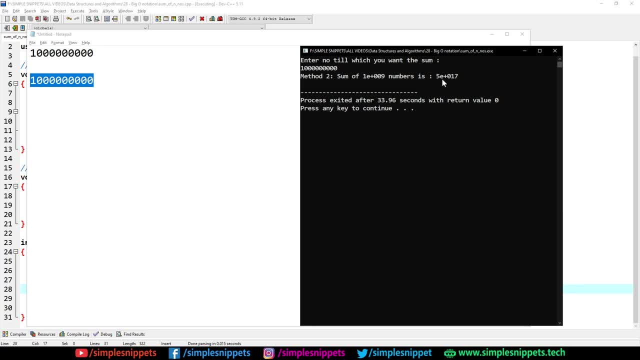 in a large weird number. don't go on the number, but you can see that when i hit enter it literally printed out the output instantly. we did not even have to wait for two seconds, but for algorithm one we had to wait for eight seconds. so you can see that this algorithm two, which is of constant time, 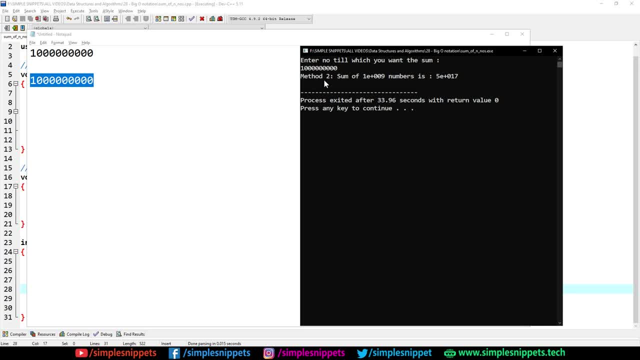 has a larger amount of inputs. so if you had to make a choice between the two, you would obviously go with algorithm number two and, by the way, they are showing us the same results. okay, so the output is correct. it's not showing some random values. you guys can put in some small numbers to see the 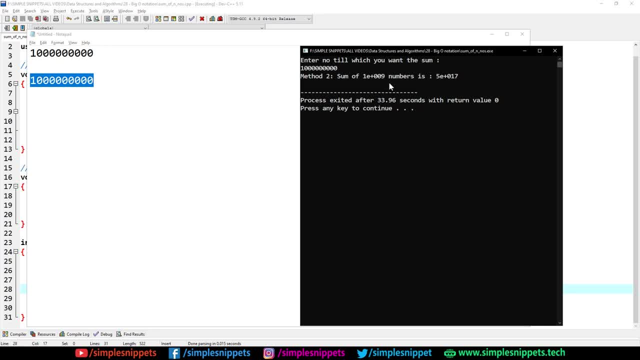 actual output. okay, that is the sum of n integers. algorithm one and algorithm two will give you the exact same numbers or exact same output. so, yes, this was a practical view or practical demo of how the algorithm time complexity changes with different algorithms which are achieving the same 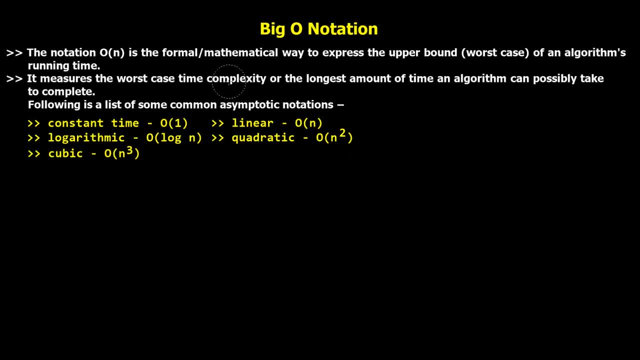 results. now let's actually switch back to the digital blackboard. okay, so now this actually brings us to the very last topic, which is one of the most important one of this entire video, which is the big o notation. so what is this big o notation? now, we just saw two different types of 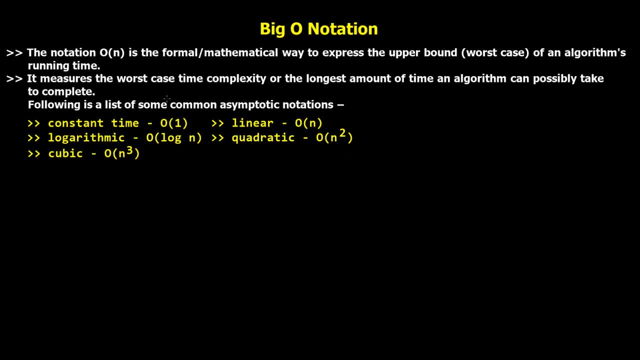 time complexities, which was linear time and constant time. now, similar to that, we have some more time complexities depending upon the behavior. so we have constant time, which we just saw, we have linear time, we have logarithmic time, we have quadratic, we have cubic and we have linear time. 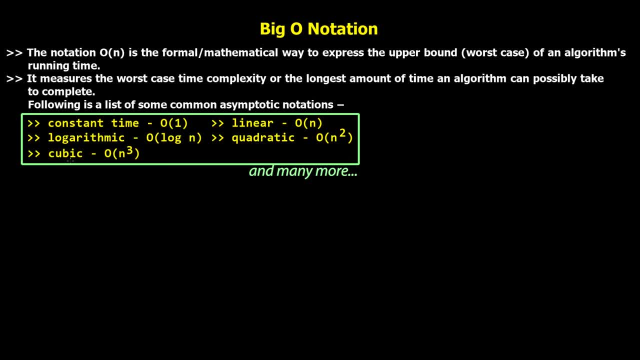 we have n number of other different types which, if you want, i'll put a link in the video description, but in order to denote them in a mathematical way, we use this big o notation. okay, so instead of telling this algorithm is linear time, or this algorithm behavior is quadratic, or this algorithm's 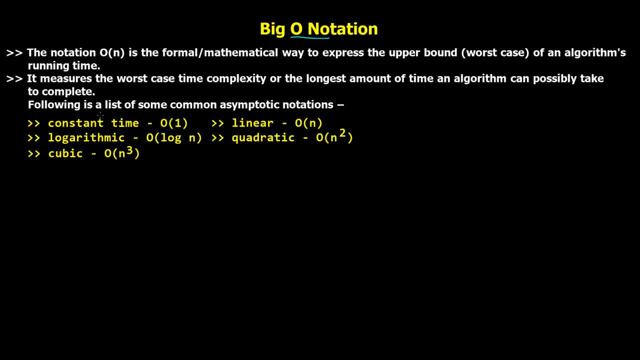 behavior is constant time. we say big o of n for linear, okay, or big o of n square for quadratic, way to express the upper bound or the worst case scenario of an algorithm's running time. so what it does is it measures the worst case time, complexity or the longest amount of time. 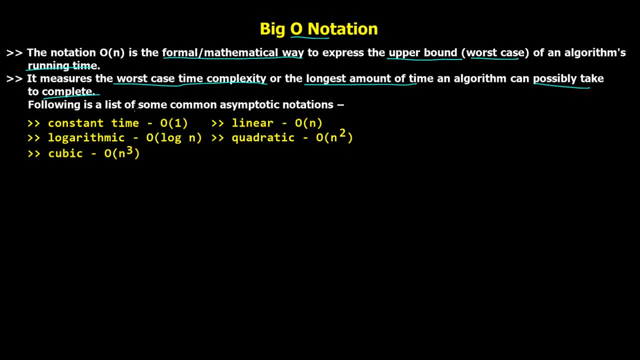 an algorithm can possibly take to complete. so now you're wondering: okay, so if big o notation is measuring the longest amount of time, what is measuring the shortest amount of time? so we have other two notations also, which is omega and theta notations, but they are not as relevant as big o. 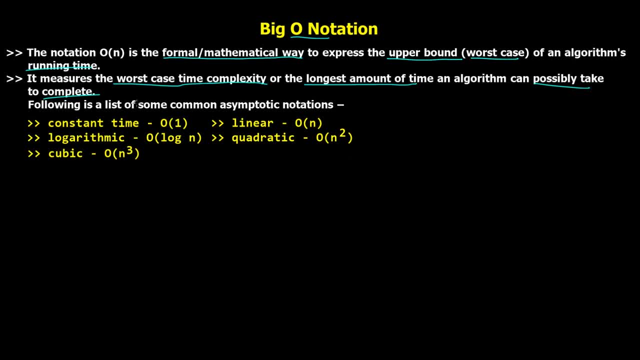 notation, because whenever you're running an algorithm, the most time you're going to be interested in- and the last important aspect when it comes to time is you want to know- is how long, or what is the maximum amount of time the algorithm will take given a particular size of the input. 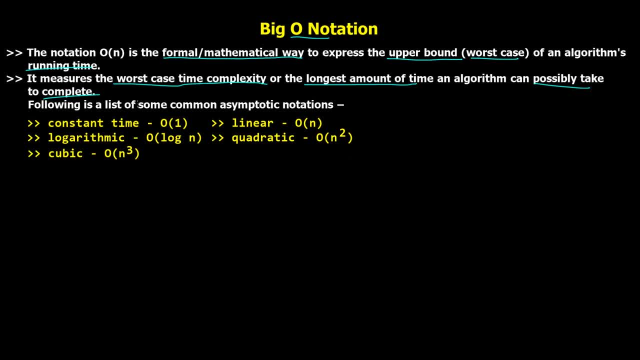 you're not worried about how fast it will execute, right, you're mostly worried about how how much maximum amount of time will it take to execute, because that is more critical. you want to know the worst case rather than the best case. if you know the worst case, you can work around all the 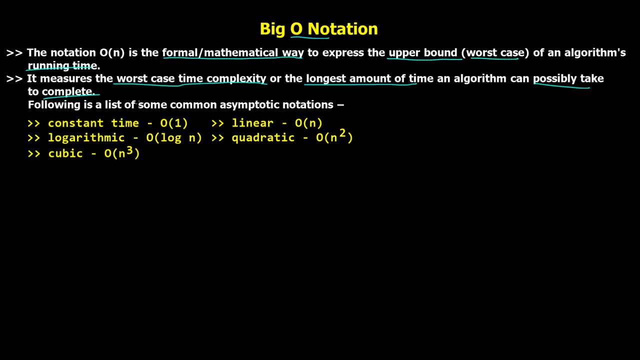 other algorithms to match that. and then you know that worst it will, your algorithm will take 10 seconds or less. so that's why big O notation is very much more important and relevant. not to say that others are not important, but big O notation is more important. so the way some asymptotic notations are is for constant time. we say O of 1, okay, you. 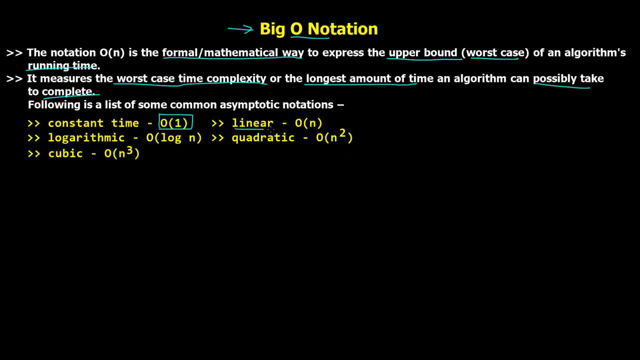 can say O of 1 or big O of 1. that's how you say it. for linear you say O of n, which means that when n increases, the time also increases. it is linear. so this is that linear behavior that we saw we are. we have one more as logarithmic, we have quadratic, which is also known as exponential. 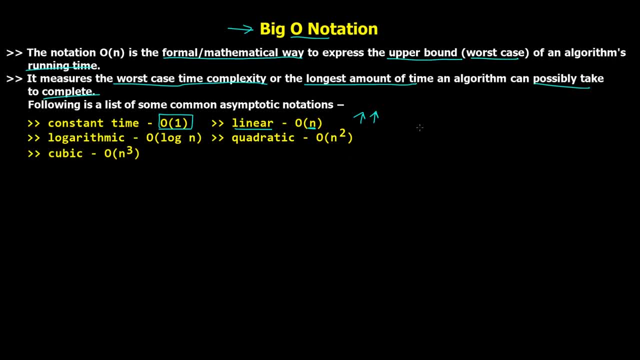 behavior. so when the n increases, the time increases the square times. so if n is 2, the time might be 4, but if n becomes 3, the time taken would be 3 square, which is 9 if it becomes 4. so n is the input size, this is n and this is the time. 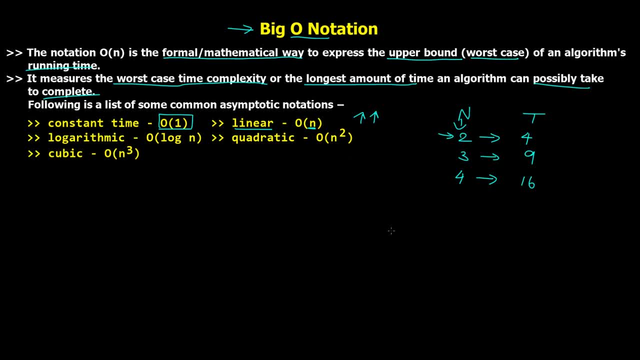 so if it becomes becomes four, four square will become 16. so on a graph, if this is n and if this is basically the time, so the graph would look something like this: okay, this would be two, this would be two somewhere over here, then we have three. we have three somewhere over here, then we'll have four. we'll. 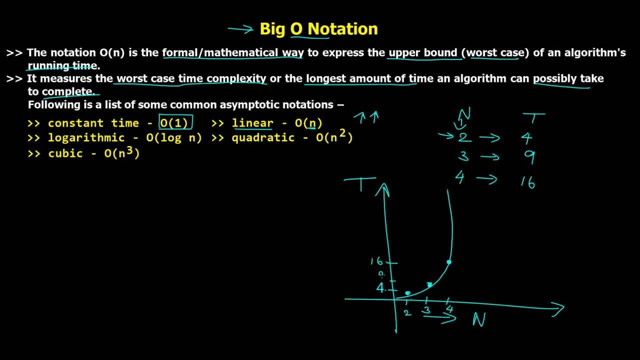 have four over here and the time is going to be 16, this is going to be nine and you can see there is an exponential growth over here. it's not linear, it's not like this. it's not a line, it's a curve. okay, this is quadratic growth or you can say it is exponential growth. now one last question: that 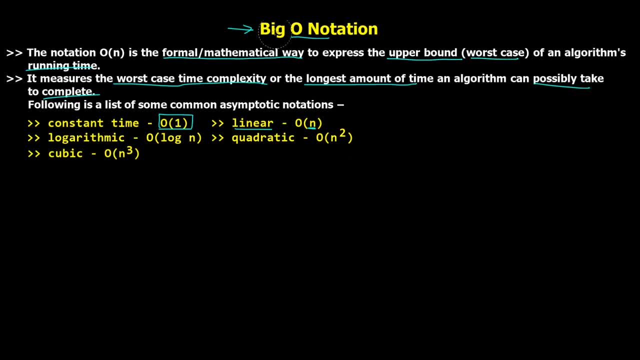 comes into our mind is: how can we calculate this big O notation? because now that we understand that big O notation is just a way to represent the time behavior of different algorithms and we are just calculating the upper bound, how can we calculate it ourselves using basic algorithm? 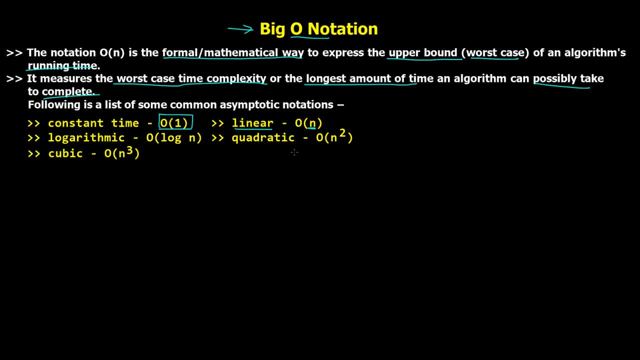 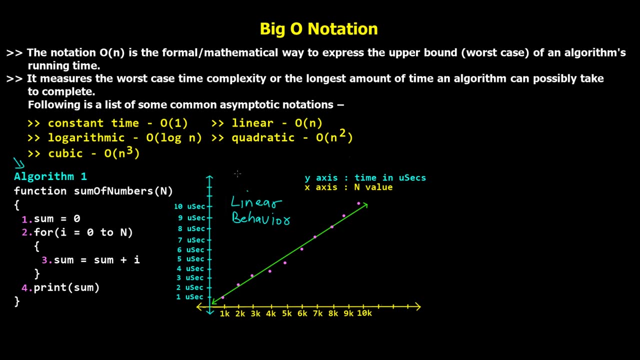 analysis right, so that is most important. So let's take our previous algorithm example itself and let's do this big O notation calculation ourselves. okay, so, as you can see, we have this algorithm, one which we just saw previously, which was having a linear time or linear behavior, and now we can also denote it as O of n or 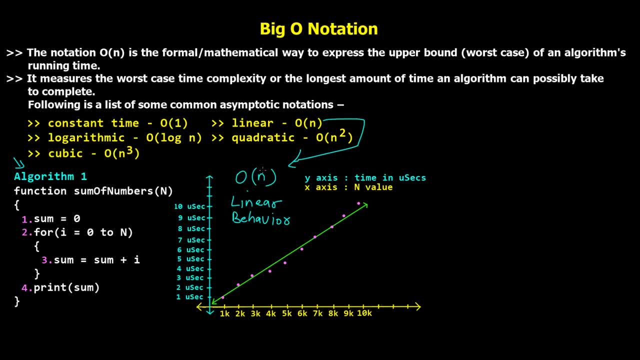 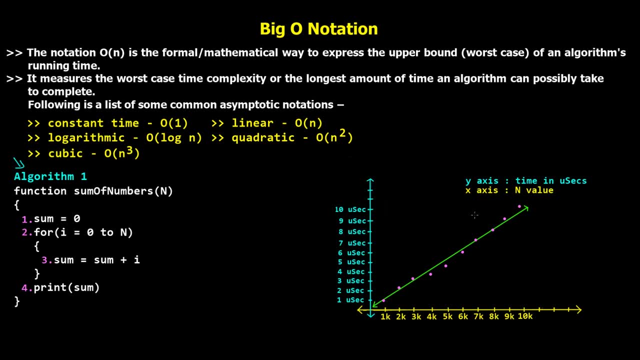 big O of n, now that we know that linear is called O of n or big O of n. but why is it called O of n? so let's try to understand that, okay? so I just shifted the graph over here. we don't really need the graph right now. we already know that it is a linear behavior. 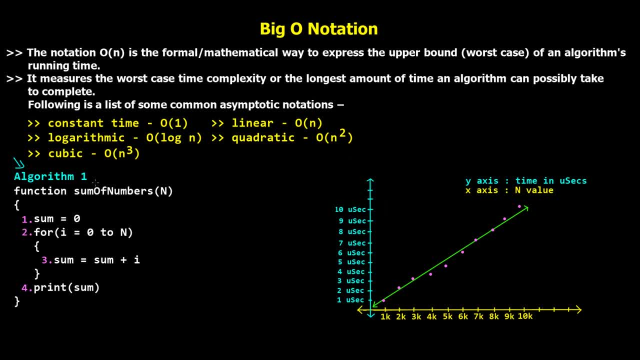 so how do you go about coming to this conclusion that algorithm one is O of n, so let's actually go step by step. so in the algorithm analysis, we know that this step is taking one microsecond, so we are making assumptions. it can be two, it can be three, but it is going to be some. 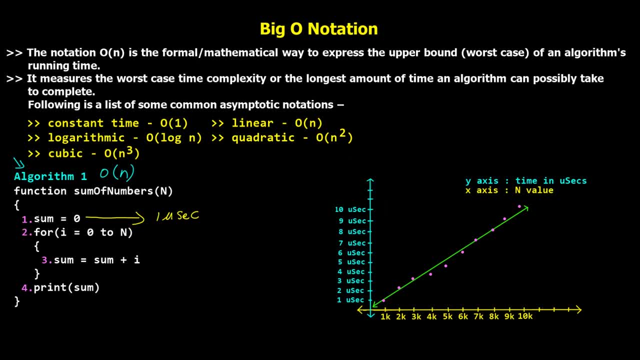 value itself, which is not going to change, right? so if this step is going to take one microseconds, it's always going to take one microseconds or something around that. for step number two, the for loop initialization, let's assume again it is taking one microsecond- the inside for loop, this step number three will run for n times, depending upon what. what 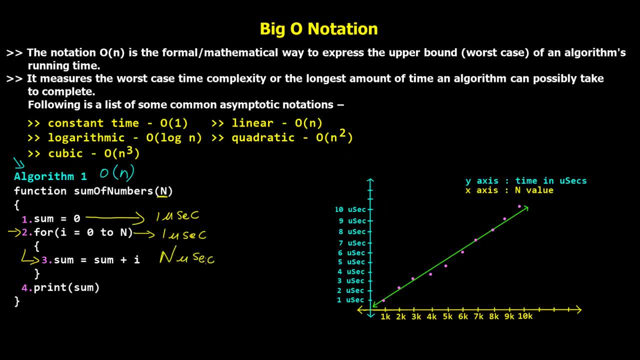 the value of n is. so I'm going to say n microseconds, so it's going to get multiplied with n. this last step again, let's assume it is taking one microseconds. so, analyzing this totally the time, let me use another color. t is equal to one plus one plus one, which is three microseconds. 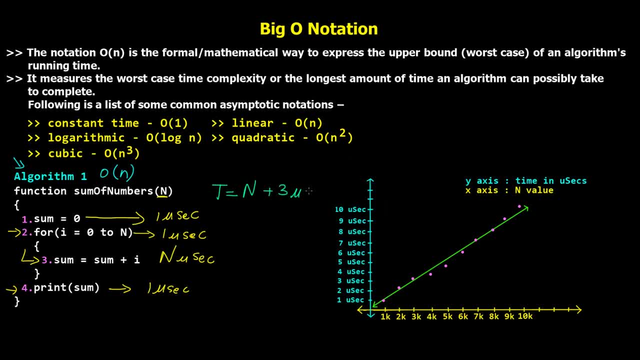 plus n, so it is going to be equal to n plus three microseconds. now the way you calculate big O notations. we have two basic steps. okay, let me just show it to you. so these are the two steps. when you want to find out big O notation by yourself. 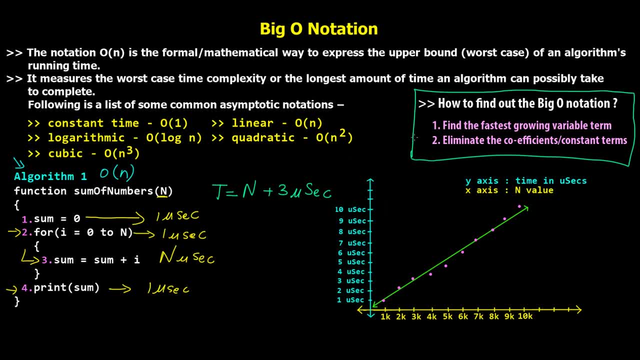 in a practical sense. so it's not exactly how a systematic way goes when it comes to calculate big O notation. that can be a separate tutorial itself. you can google it out also, but in a practical sense you can also do it yourself just by studying the entire algorithm and 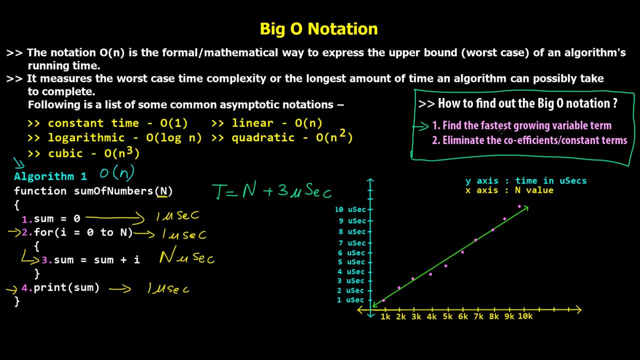 the two major steps are. first thing is we have to find out the fastest growing algorithm, the fastest growing variable term in the entire equation. now this has become an equation for time complexity, so this t is representing the time complexity. so in this equation we have two terms. this is the first term, then we have a plus in between and this is the. 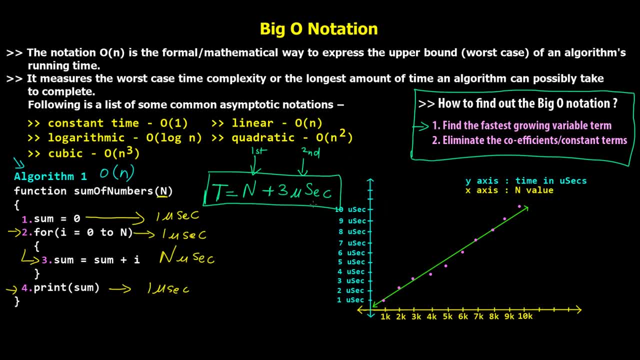 second term. now, looking at this, you can say that this three microseconds will never change, whatever the n value. this three microseconds is because step number one, two and four always takes one microseconds, so this can be considered as a constant, right? so I'm going to write constant over here. however, if you see, this n is actually a variable because it keeps. 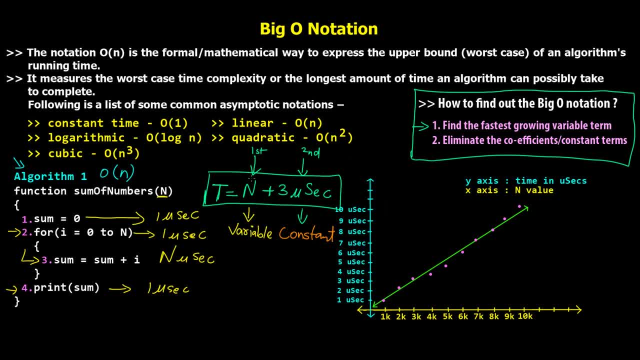 on changing. so we have to find the fastest growing variable. we only have one variable in this entire equation, right in on the RHS of this entire equation, so as whatever value of n you put, the time also increases, because it is a linear behavior which all which we 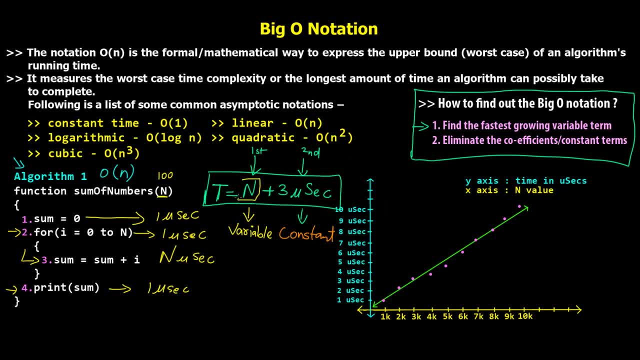 already saw. so this is the fastest and this is actually the only variable right. so we found the variable. so what is step number two? step number two is you have to eliminate the coefficient of the variable Efficient and the constant terms. so over here, the only constant term is this: which? 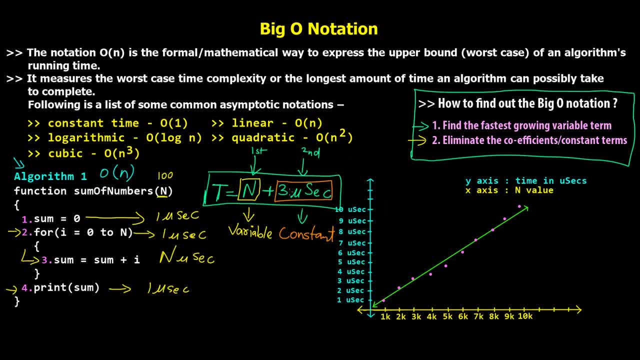 is the extra time required for these extra steps, but they will always take some constant time, so that is the constant term. so what is this coefficient? so the coefficient can be some value attached with this n. okay, right now we don't have any value, but it could be. 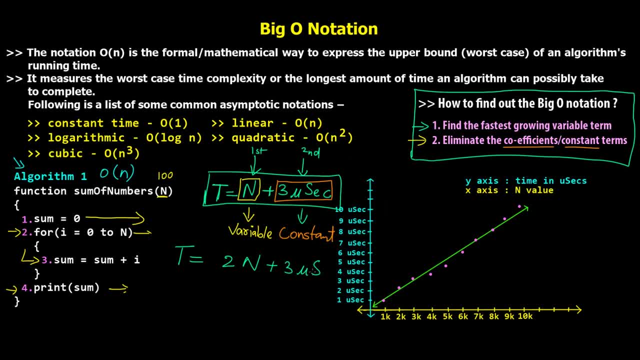 something like p is equal to 2n plus 3 microsecond. now this two is essentially a coefficient. okay, it's a coefficient. n is a variable and this component is a constant. so what we have to do, we have to find the fastest growing variable, which is n. so we found that and we have to eliminate all the other coefficients. 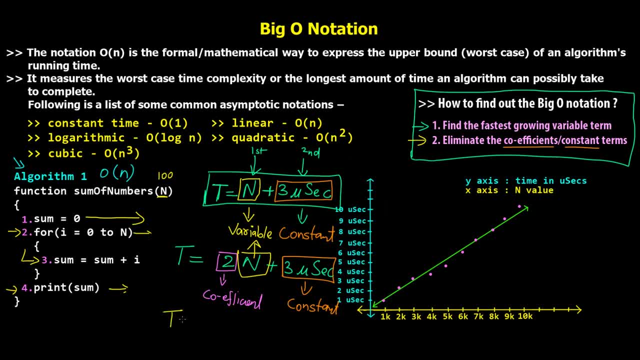 and constants. so ultimately, the time complexity t will be equal to n, right, and it is also denoted as o of n or o of capital n or whatever the value over here. what is more important is the term that we are left with. we took capital n, so it would be o of capital n, okay, so this is the time complexity. 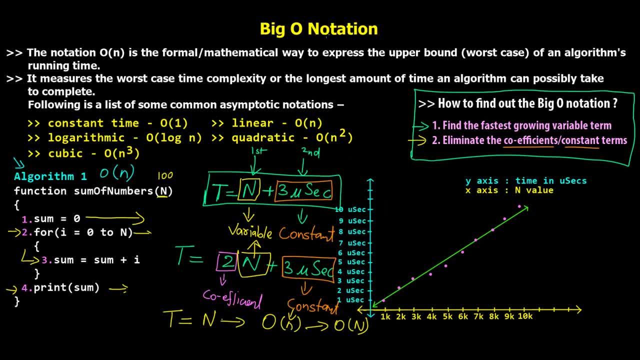 which is o of n. so this is how you found out the big o notation for this algorithm, which is basically having a linear time behavior, which is represented by o of n. now, quick note: these constants and these different coefficients can be added in any algorithm because, as i mentioned, 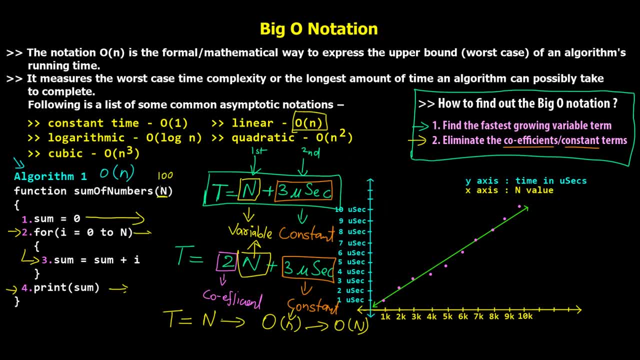 whenever an algorithm is running in your system, it is not just dependent upon the time complexity that we are left with. we took capital n, so it would be o of capital n, the number of steps. it is also dependent upon how fast is your processor, how fast is your ram, what? 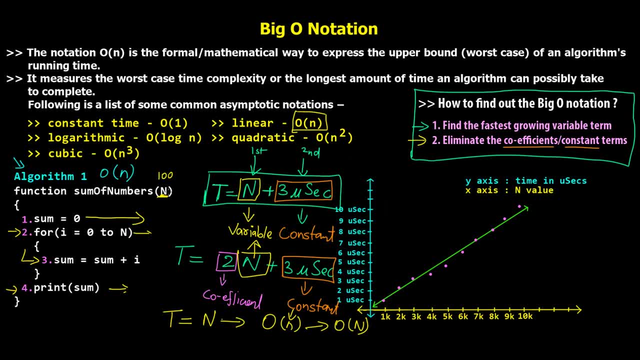 is the size of your ram? is your processor 7 gen? is your processor 9 gen, right? what is the cpu speed of your processor? so all those things, basically are these coefficients and constants which get added to this entire equation, and then, ultimately, we just have to figure them out and just focus on. 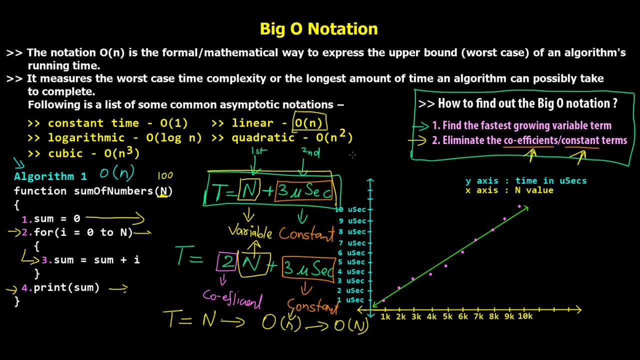 the fastest growing variable. sometimes in an equation you have multiple variables also. so when it comes to quadratic kind of equations, it would be something like: t is equal to n square plus 2n, and so on and so forth. so in that case, which is the fastest growing variable? obviously? 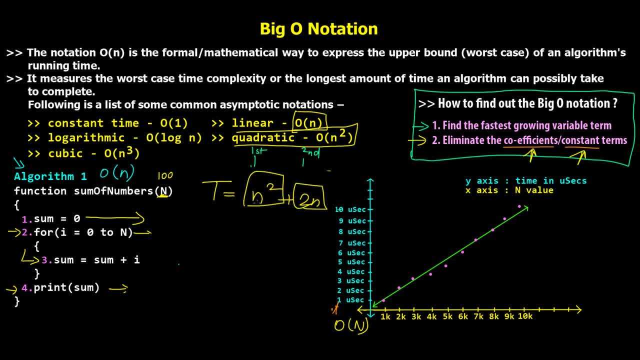 n square will grow faster than 2n when the n is very large. right, because we are doing asymptotic analysis when the input size is very large. we want the worst case scenario, so in that case we have to eliminate this part and we just focus on this n square variable and ultimately we will end up with o of n square. so 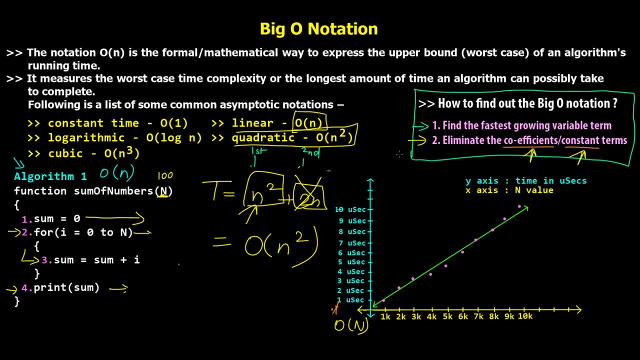 i hope you are understanding how we calculate big o notation by ourselves in a practical sense. and big o notation ultimately is nothing but a formal or mathematical way to express the upper limit of an algorithm's running time. so yeah, this was the entire video on time complexity, big o.